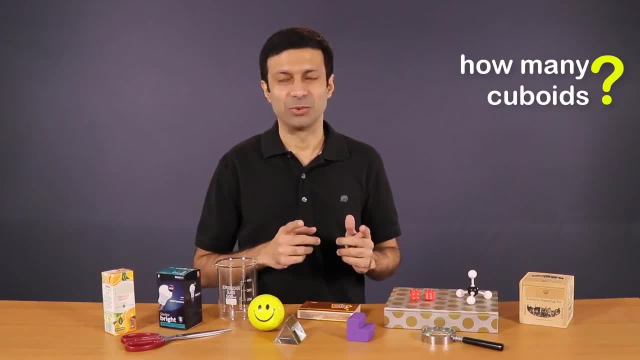 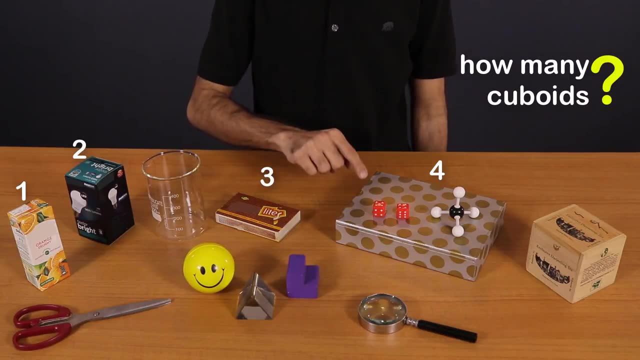 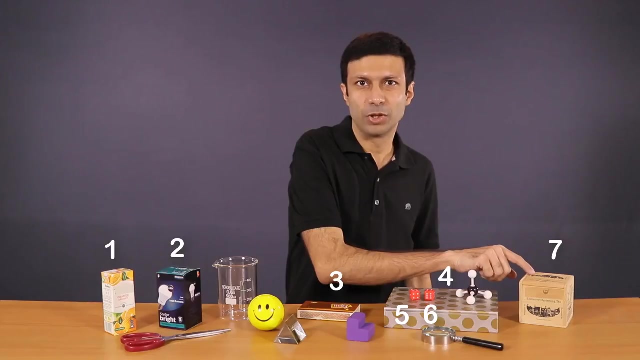 So how many cuboids are here? Let's count 1,, 2,, 3,, 4,, 5.. A cube is also a cuboid. 6 and this cube is also a cuboid, So that's 7.. 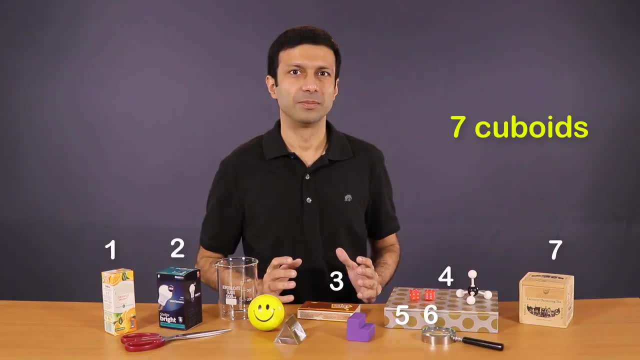 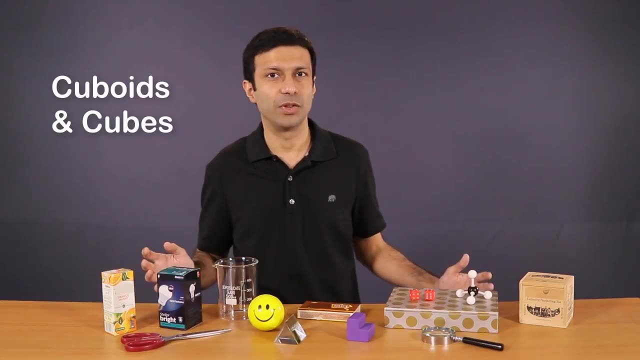 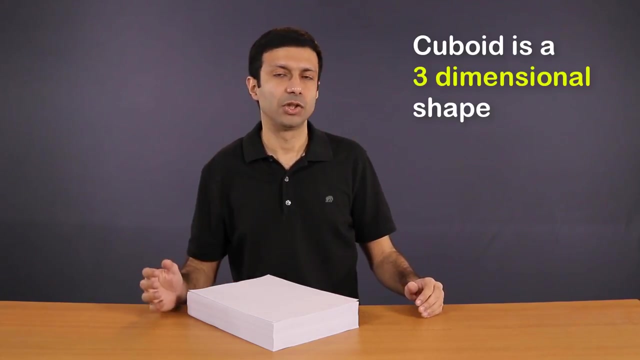 So we have 7 cuboids on this table. In this video we'll be discussing cuboids and cubes And then we'll finish the game, And then we'll finish off with our top 3 exam oriented questions on this topic. Cuboid is a 3 dimensional shape. Now what does this term dimension mean? 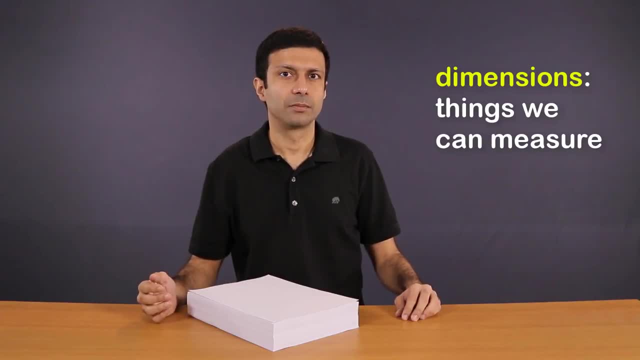 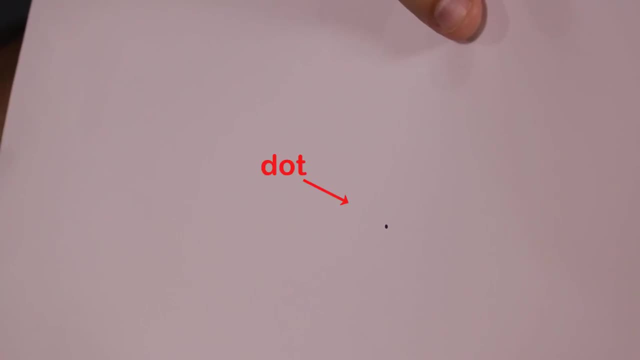 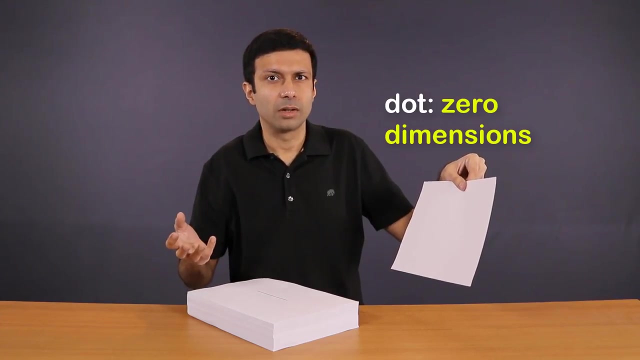 Dimensions are the things that we can measure. Let's take a look at some examples On this paper. here I have a dot. Now a dot has no dimensions. We can say a tiny dot or a thick dot, But usually we are not bothered in measuring its size. 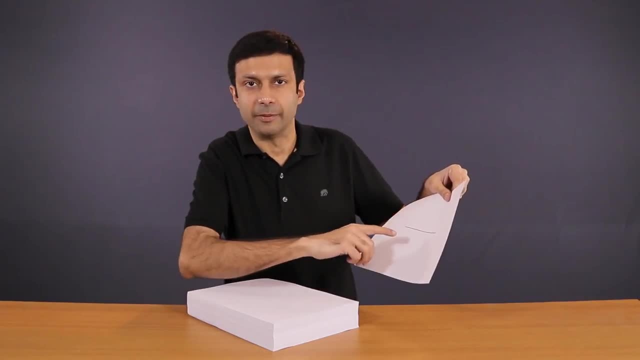 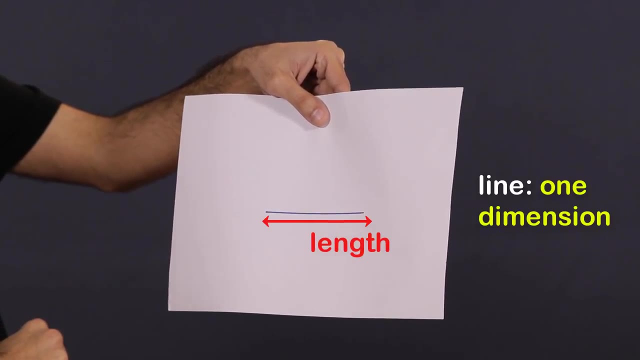 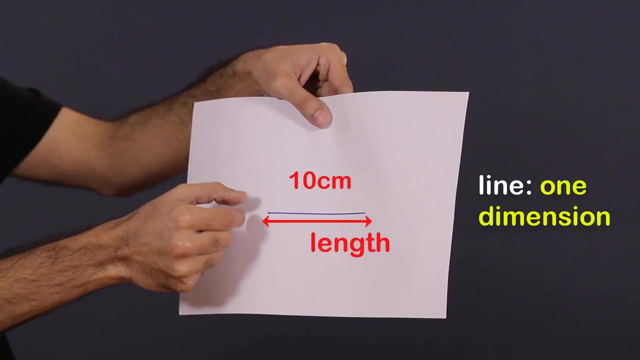 On the next paper. here I have drawn a line. A line has one dimension: its length. We can measure the length of the line. here It's going to be 10 centimeters, But we don't care about the thickness of the line. 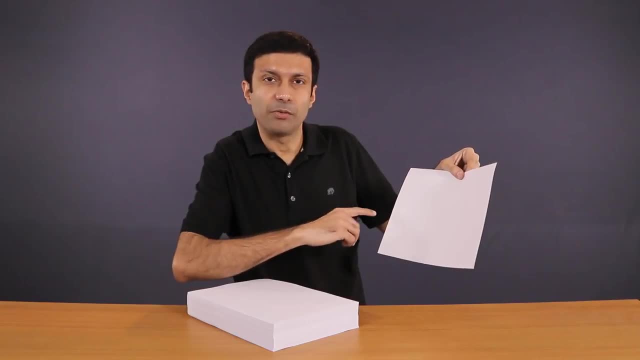 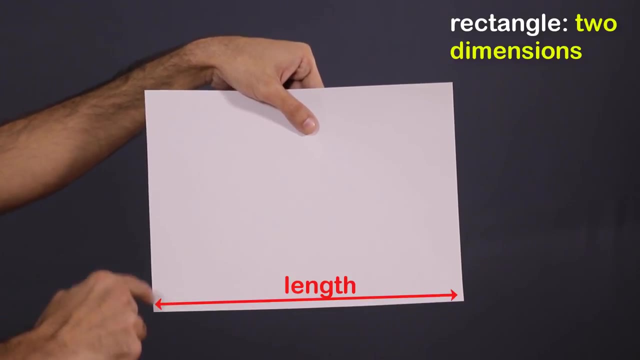 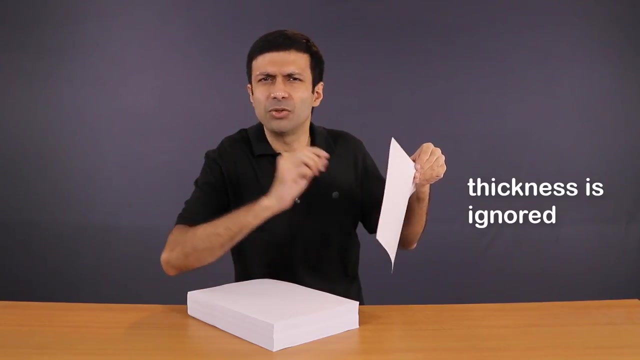 If you look at the whole sheet of paper, it has the shape of a rectangle. A rectangle is 2 dimensional because it has a length and breadth which we can measure. The paper also has a thickness, but it's really really small and we usually don't bother about it. 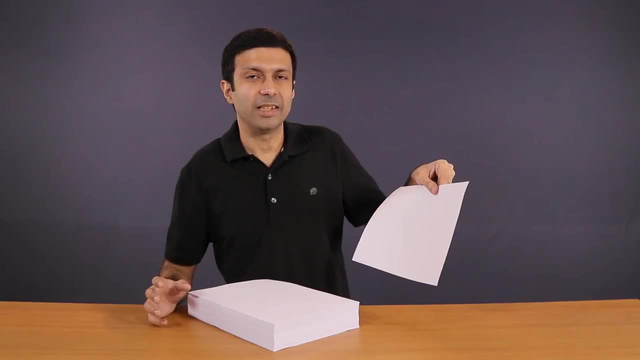 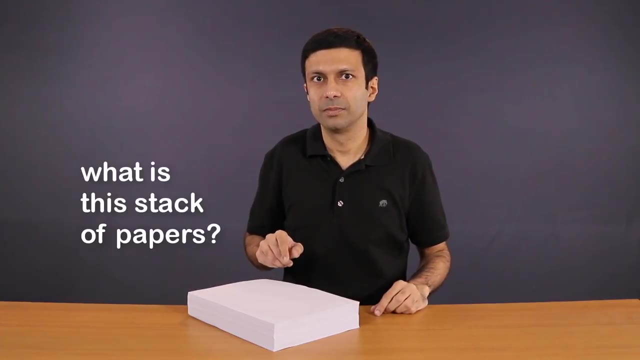 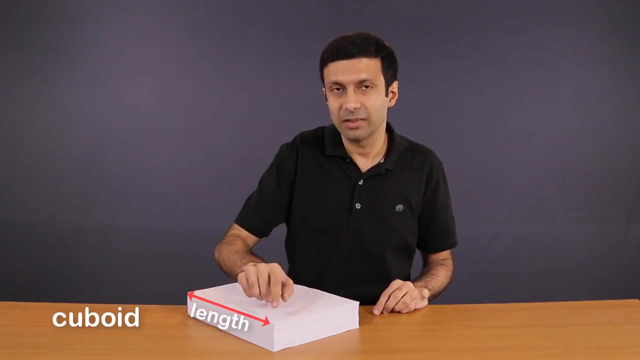 So this paper is a rectangle and it's 2 dimensional. Now, if we stack up all the papers like this, what do we get here? We get a 3 dimensional figure, Because this is a cuboid having a length, breadth and height. 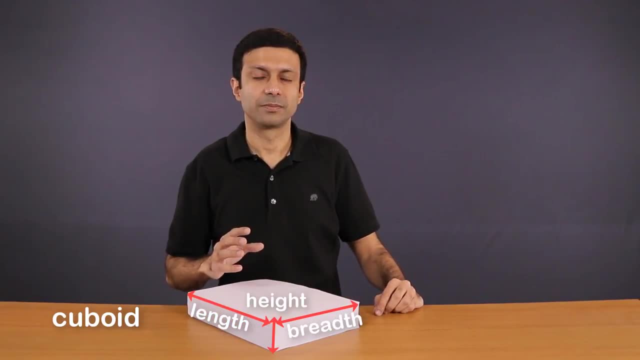 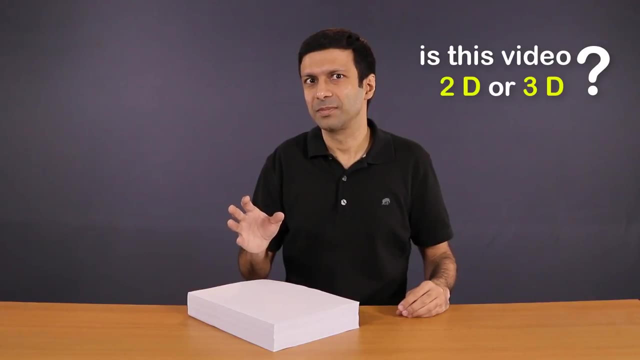 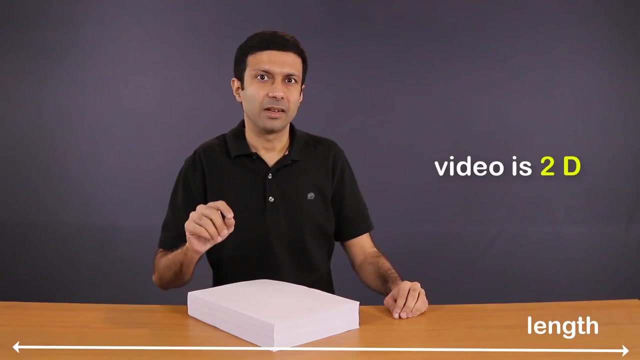 So it's a 3 dimensional object. Now, this video you're watching, Is it 2D or 3D? That's right, it's 2D, since you're watching it on a screen. It has a length and breadth but no real depth. 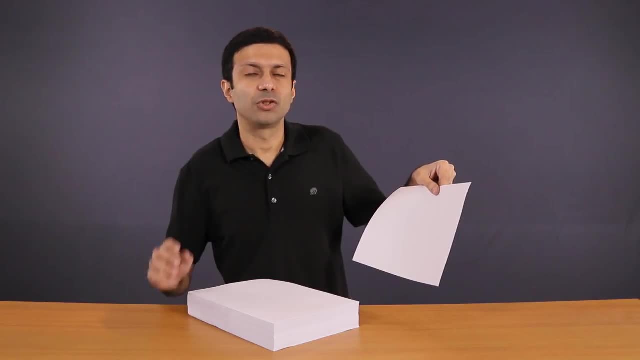 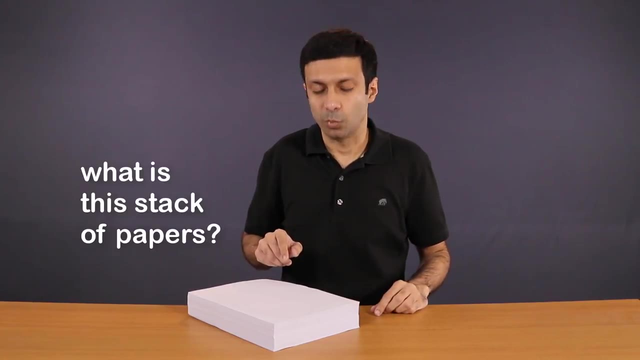 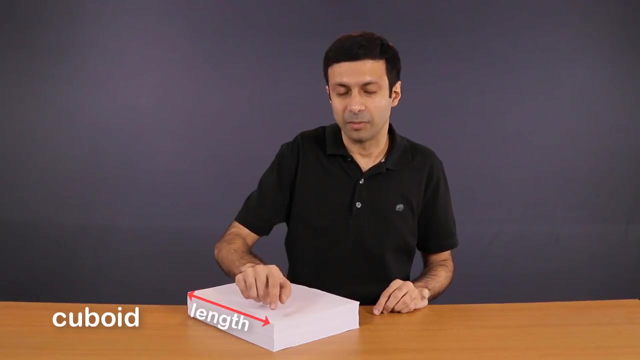 So this paper is a rectangle and it's two dimensional. Now, if we stack up all the papers like this, what do we get here? We get a 3 dimensional figure, Because this is a cuboid having a length, breadth and height. 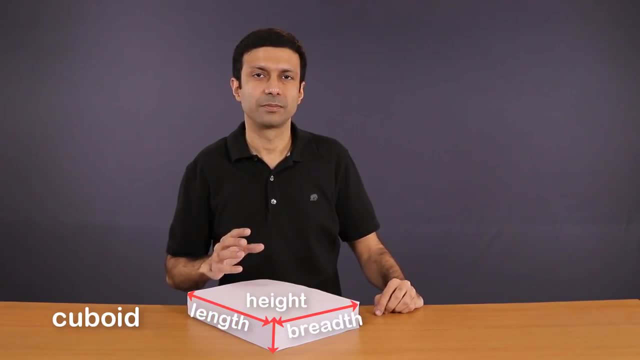 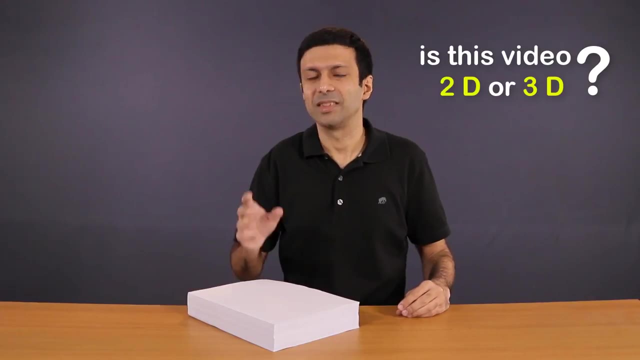 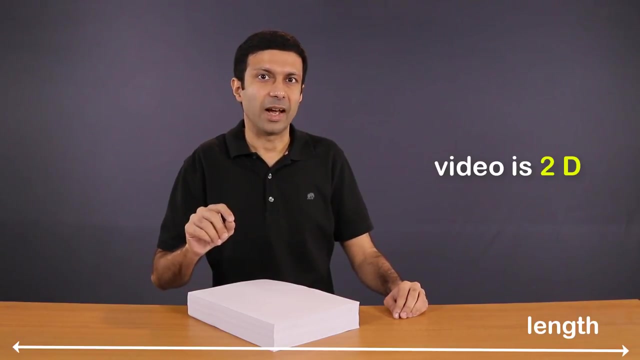 So it's a three-dimensional object. Now, this video you're watching, is it 2D or 3D? That's right, it's 2D, since you're watching it on a screen. It has a length and breadth but no real depth. 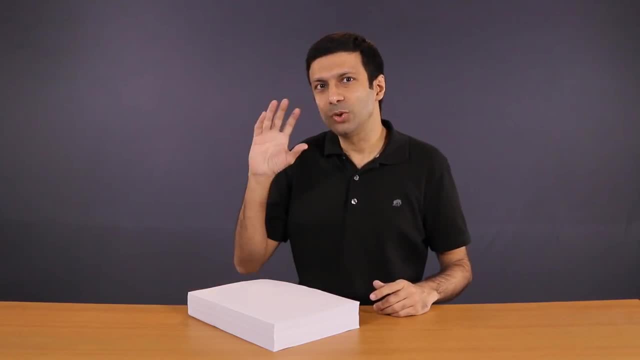 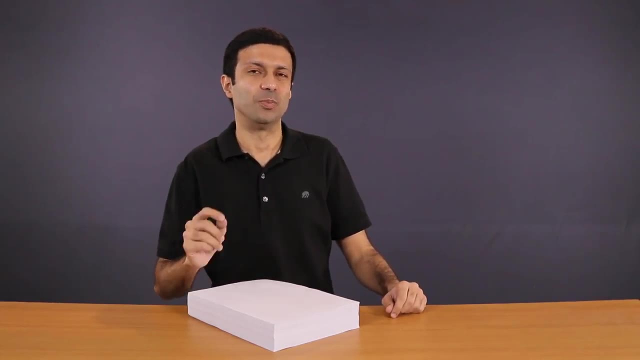 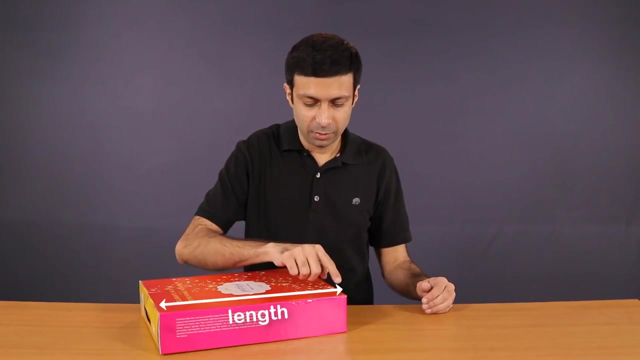 But for this video, I want you to think in 3D, since we're going to be talking about three-dimensional shapes, cuboids and cubes, As we discussed, a cuboid is a three-dimensional shape having a length, breadth and a height. 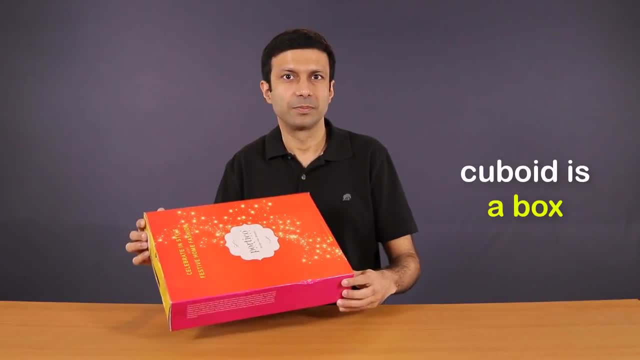 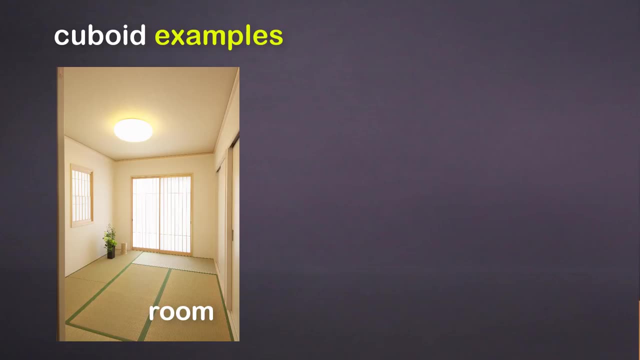 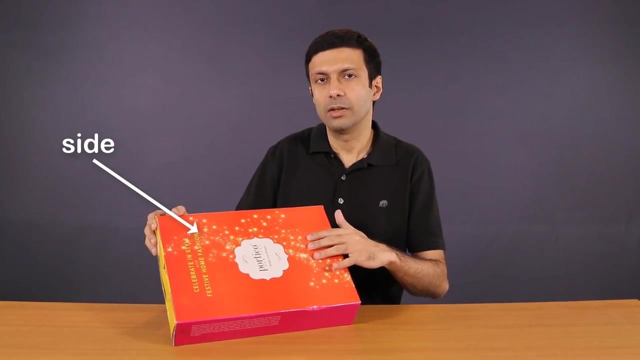 Or simply put, a cuboid is a box. Now, what are some other examples of cuboids? Your room is a cuboid, So is a book or a brick. Each side of the cuboid is called a face. So how many faces does a cuboid have? 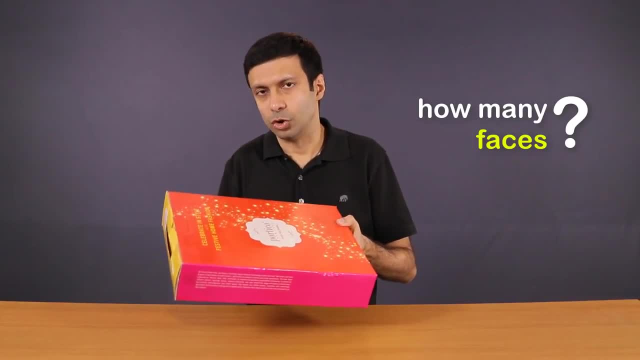 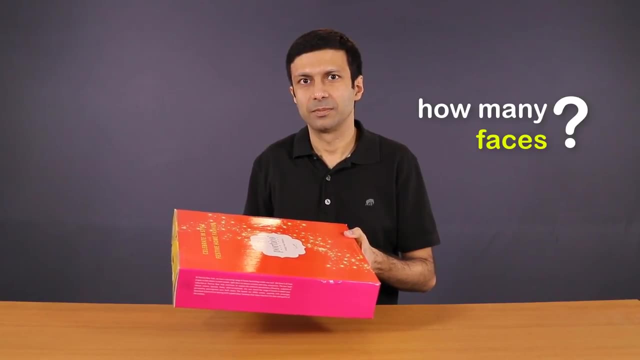 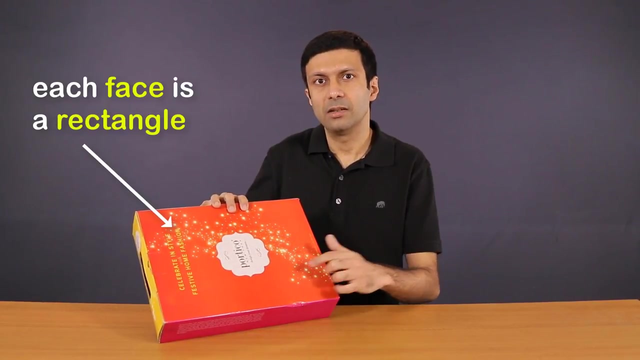 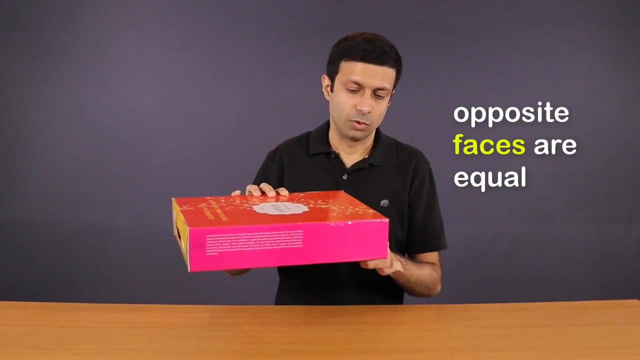 Let's count. One, two, three, four, five and six. So, a cuboid has six faces. Each face of a cuboid has five faces. � you can see, is a rectangle. And opposite faces are equal. So if you look at any 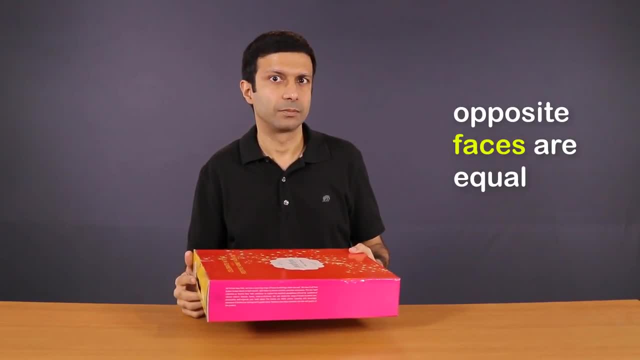 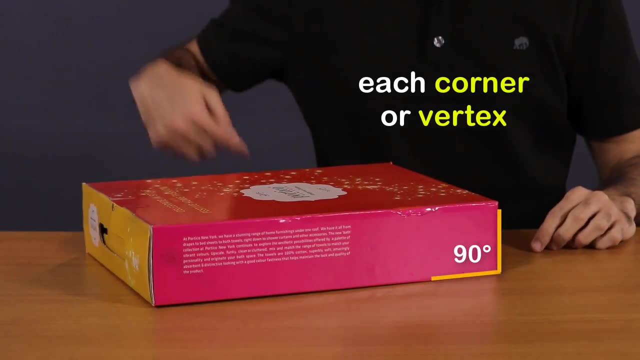 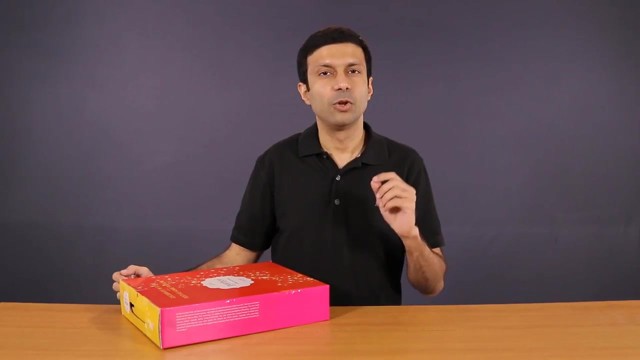 opposite face. they are equal to each other And each corner or vertex of the cuboid has an angle of 90 degrees. We can measure the surface area and volume of a cuboid. Let's look at surface area first. Surface area is the area that you can. 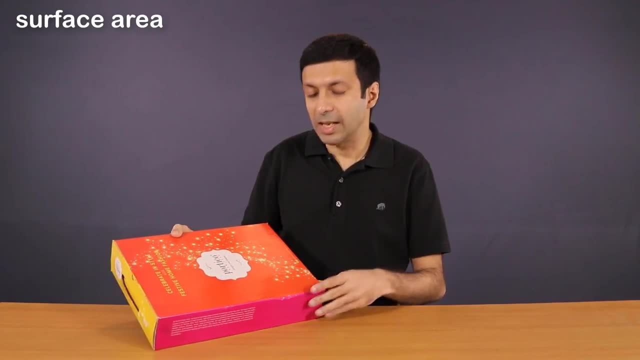 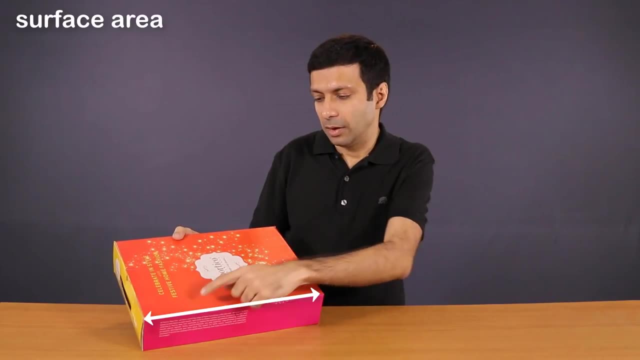 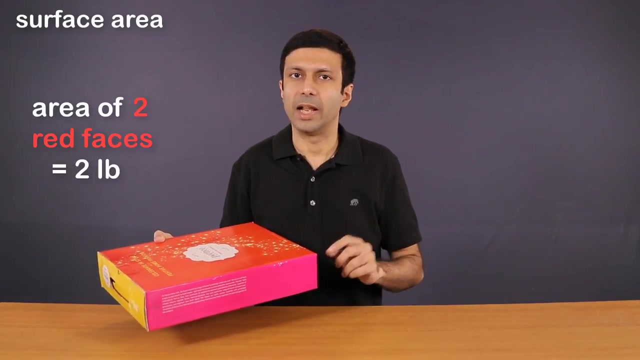 feel or touch. So let's calculate the total surface area of this cuboid. The area of the top is going to be L into B, So is the area of the base. So the sum is 2LB. Now what is the area of these two yellow faces? 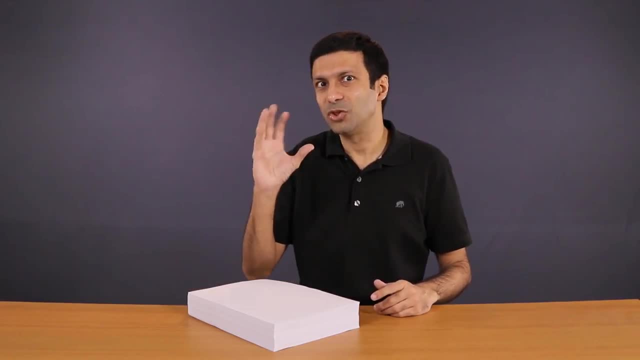 But for this video, I want to measure the length. Now, this is a cuboid. This is a cuboid having a length, breadth and height. I want you to think in 3D, since we are going to be talking about three-dimensional shapes, cuboids and cubes. 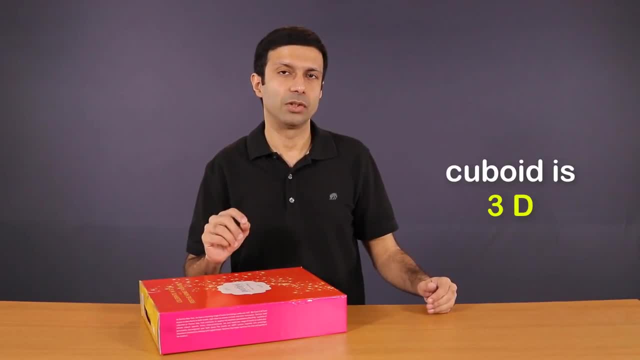 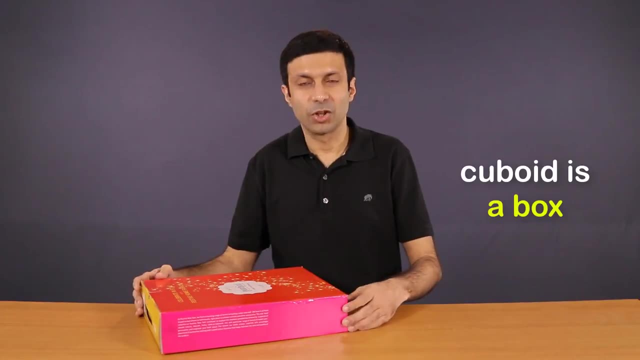 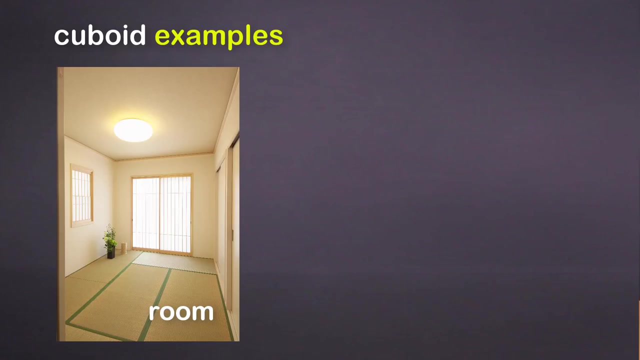 As we discussed, a cuboid is a three-dimensional shape having a length, breadth and a height, Or simply put, a cuboid is a box. Now, what are some other examples of cuboids? Your room is a cuboid, so is a book or a brick. 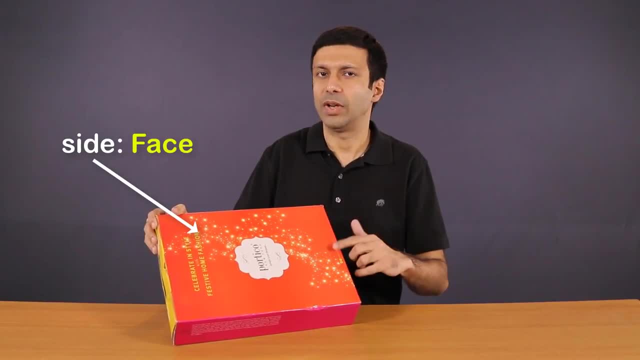 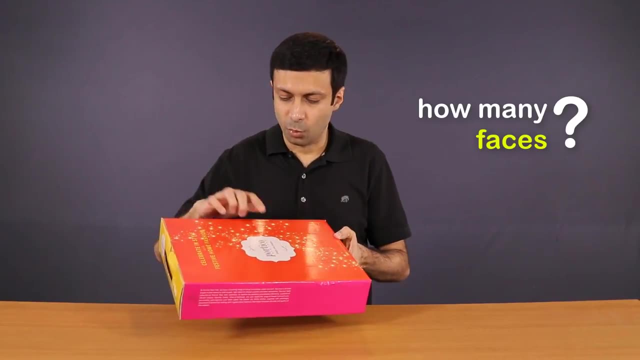 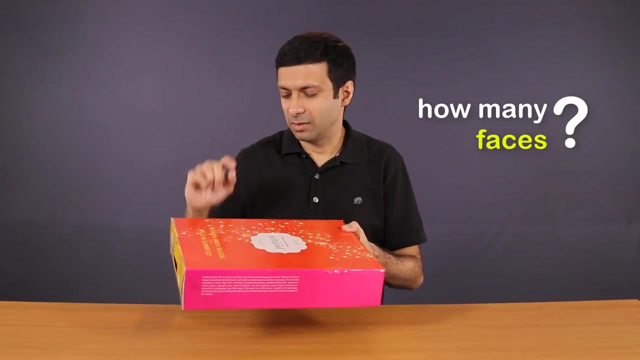 Each side of the cuboid is called a face. So how many faces does a cuboid have? Let's count 1,, 2,, 3,, 4,, 5 and 6.. So a cuboid has six faces. 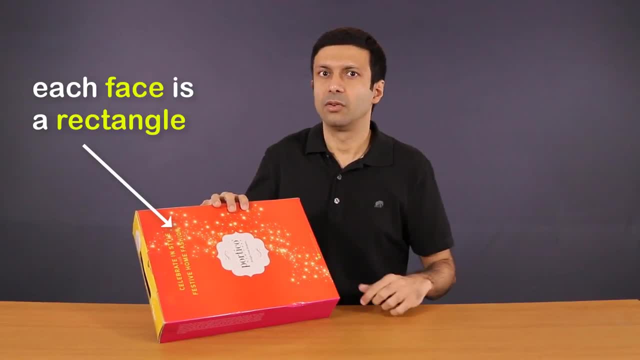 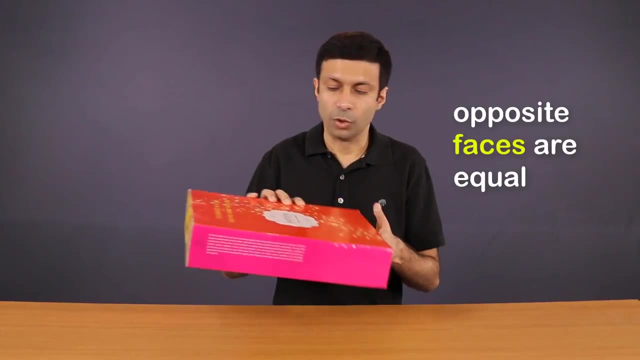 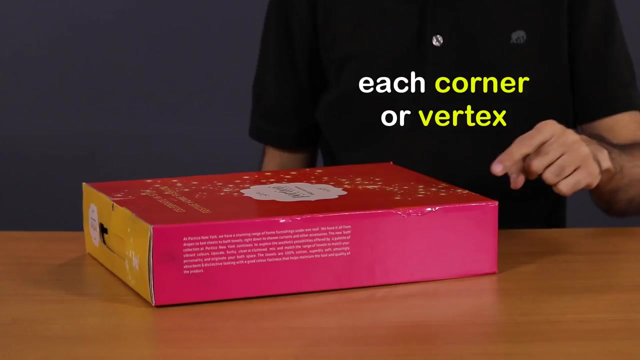 Each face of a cuboid, as you can see, is a rectangle And opposite faces are equal. So if you look at any opposite face, they are equal to each other And each corner or vertex of the cuboid has an angle of 90 degrees. 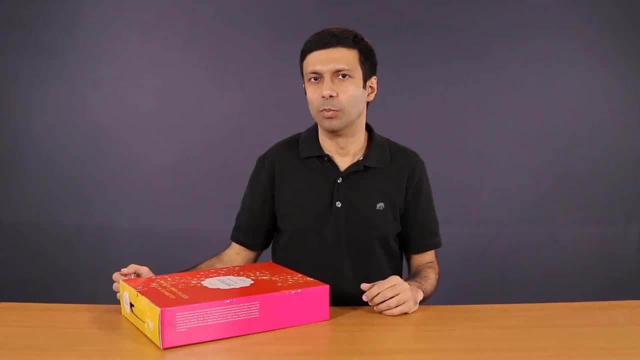 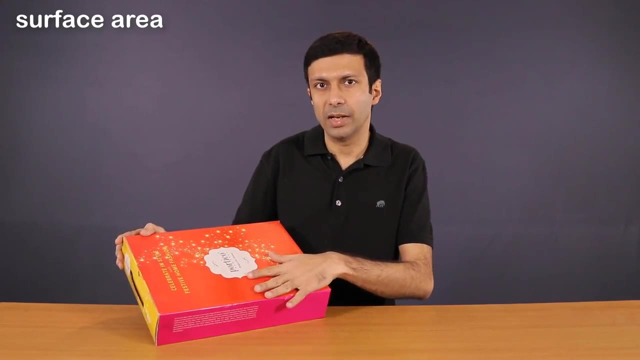 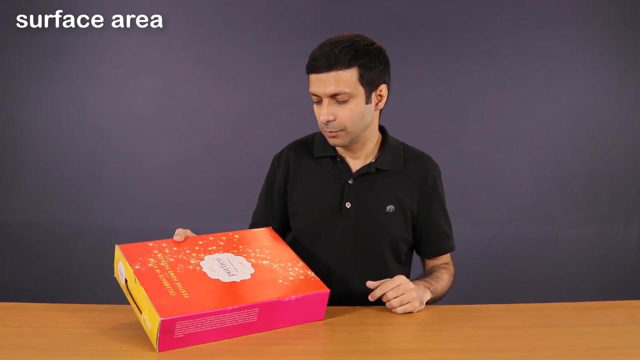 We can measure the surface area and volume of a cuboid. Let's look at surface area First. surface area is the area that you can feel or touch. So let's calculate the total surface area of this cuboid. The area of the top is going to be L into B. 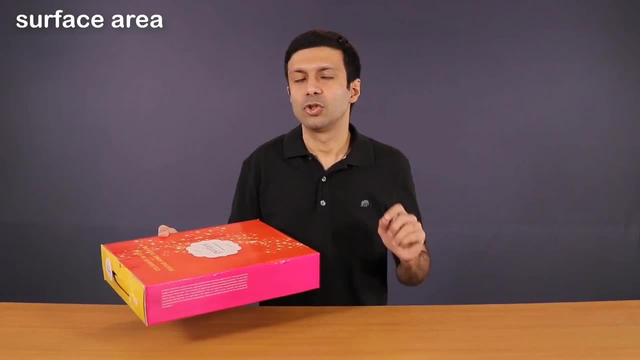 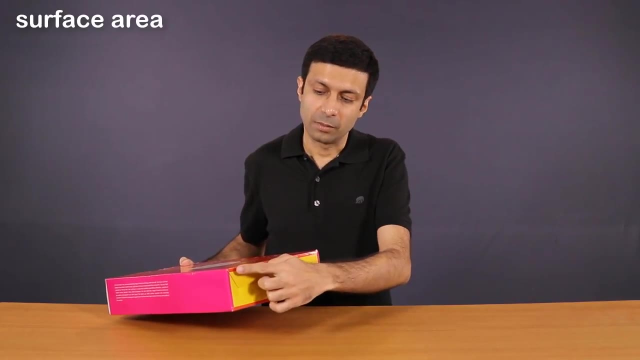 So is the area of the base. So the sum is 2LB. Now what is the area of these two yellow faces? It's going to be B into B, So the area of the top is going to be L into B. 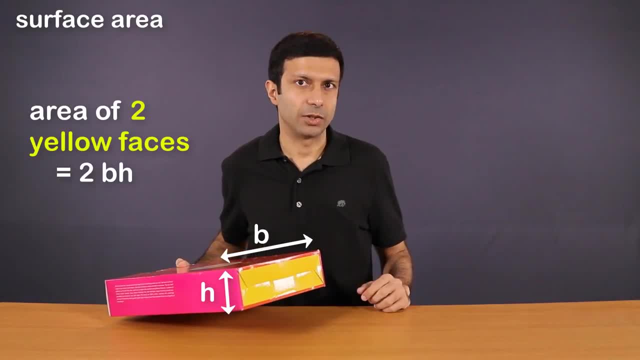 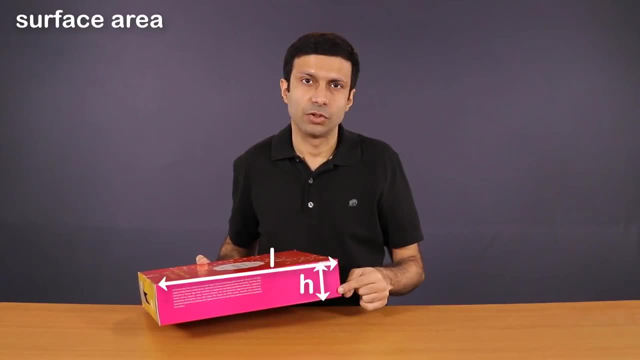 So the area of the base is going to be L into B, So the area of the top is going to be L into H, So the sum is 2BH And the area of the pink face is going to be L into H. 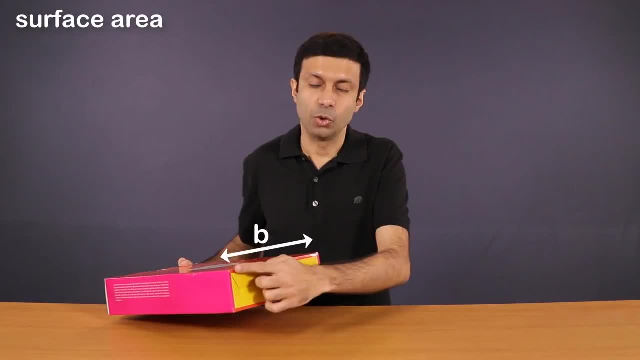 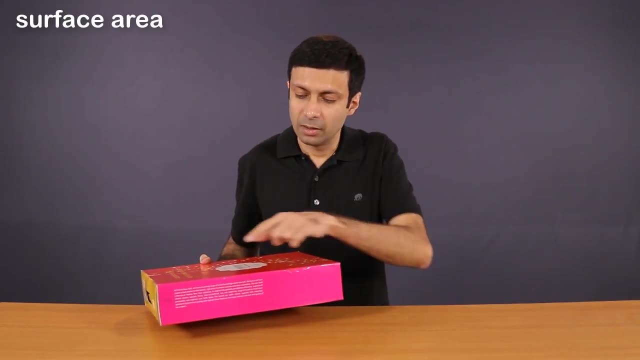 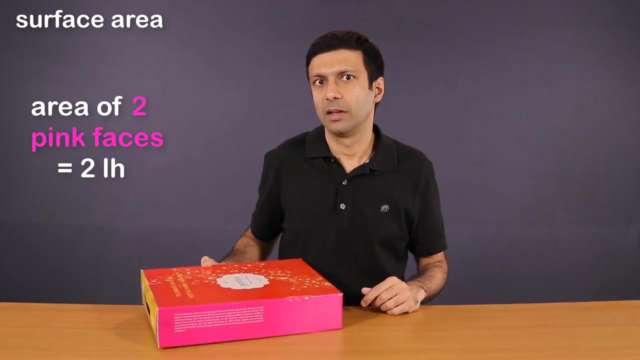 It's going to be B into H, So the sum is 2BH, And the area of the pink face is going to be L into H, So that's 2LH. So the total surface area is going to be 2LB. 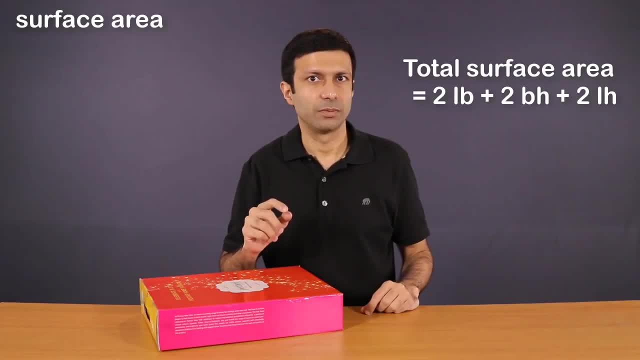 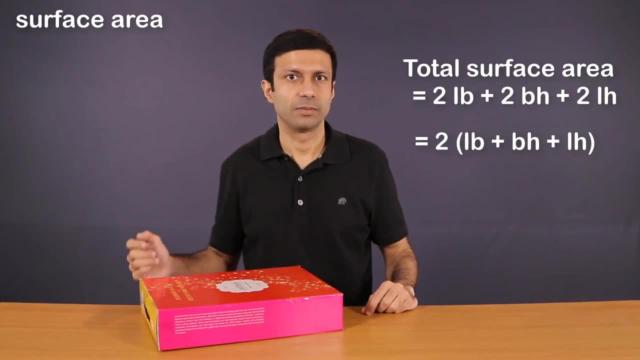 plus 2BH plus 2LH, So that's 2 into LB plus 2LH, So the total surface area is going to be 2BH plus 2LH. There's another term called lateral surface area- An easy. 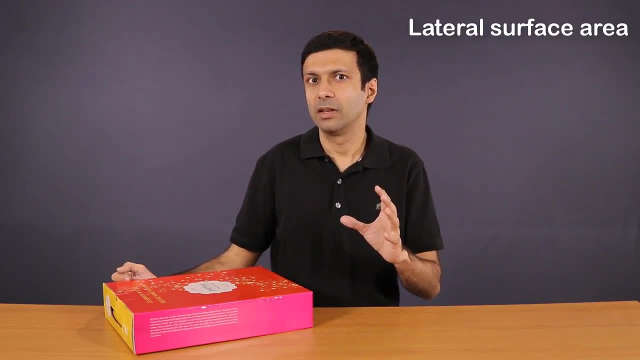 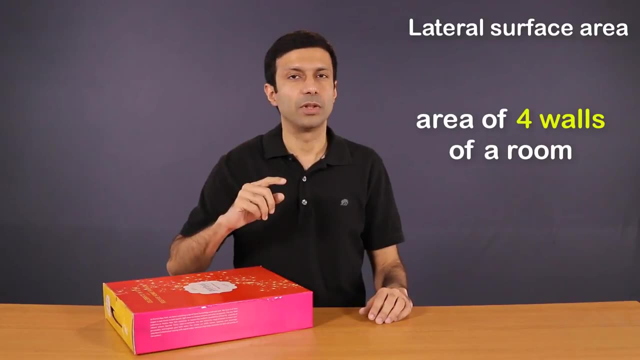 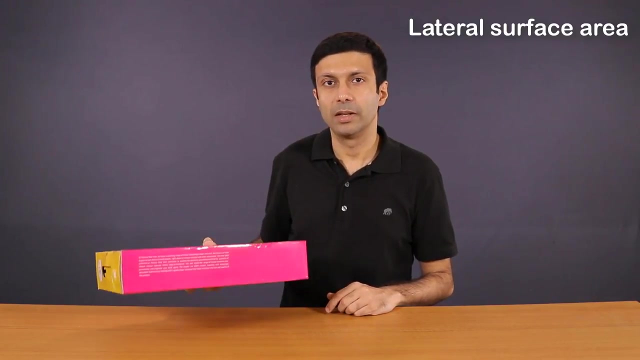 way to remember it is that the lateral surface area is the area of the four walls of your room, So not including the area of the ceiling and of the floor. Now, what will be the lateral surface area of the cuboid here? It's going to be the sum of the area of these two pink 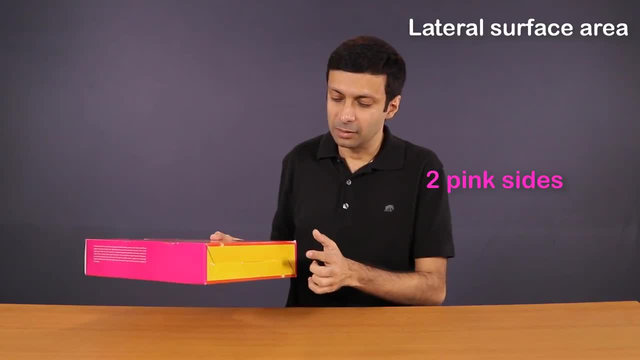 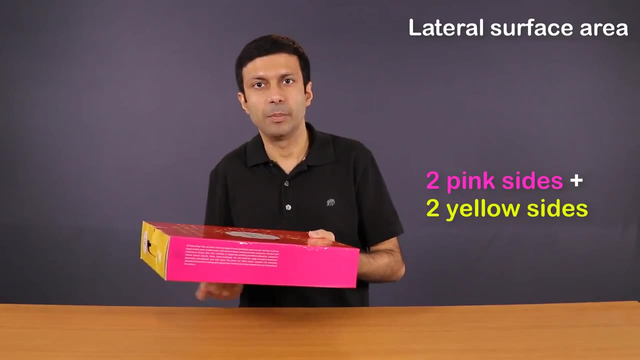 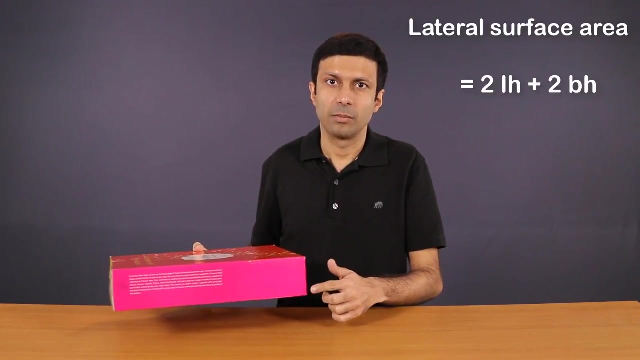 sides, So these two And the sum of the area of these two yellow sides. So I'm not including the top and the base here. So what will be the formula? It's going to be 2LH plus 2BH, So that's 2H into. 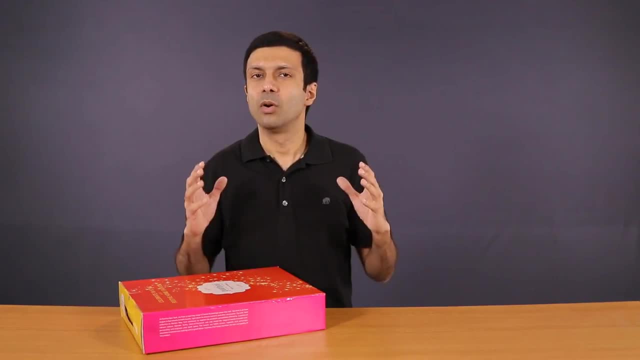 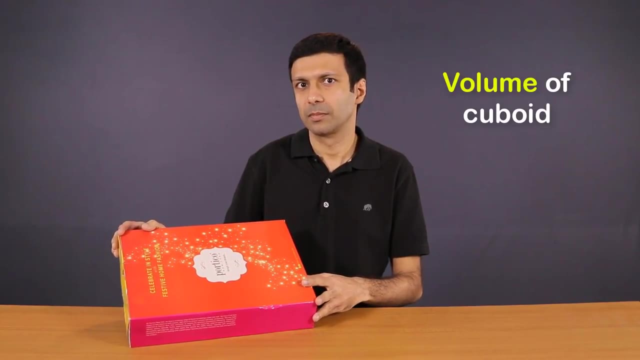 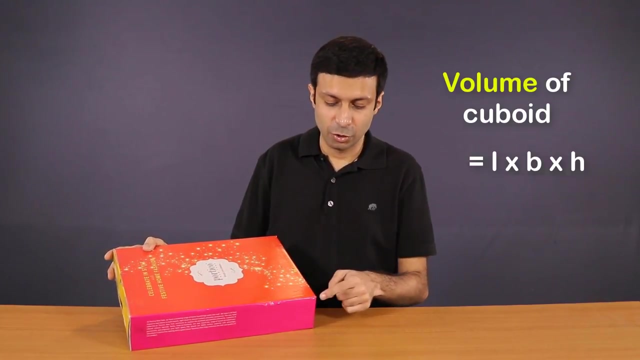 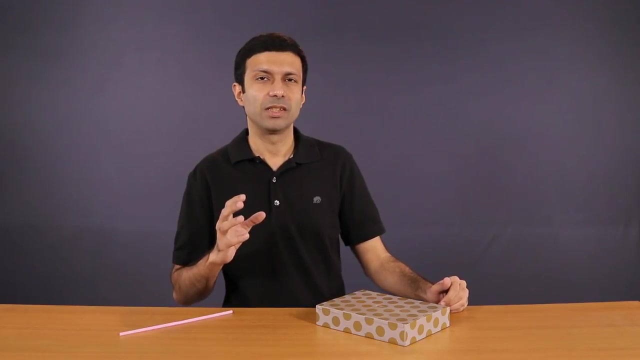 L plus B, We can also measure the volume of a cuboid. Volume means the space that this box occupies. So what is the formula for volume? It's going to be length into breadth, into height, So the formula is LBH. Now an interesting question is: what is the longest? 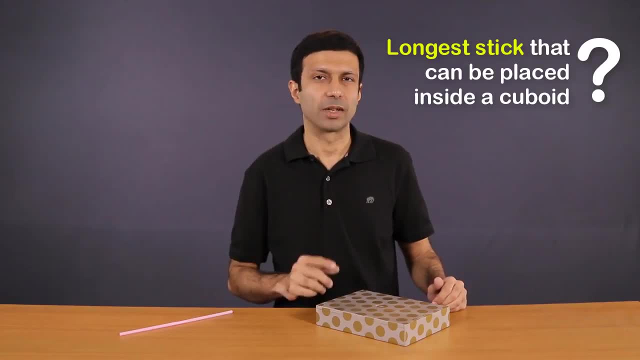 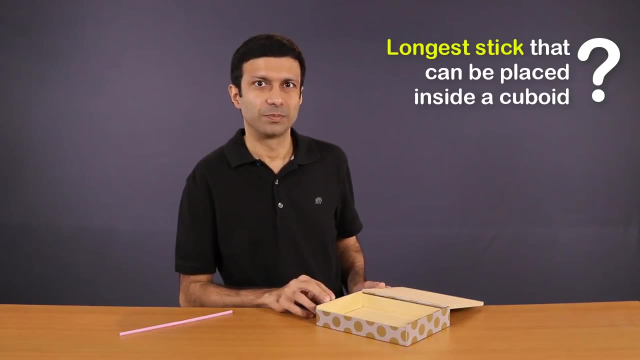 stick that we can place inside a cuboid or a box. Here I'm using a different box because it's easy for me to open this one and show you. So let's go ahead and try it. So let's go ahead and try it. 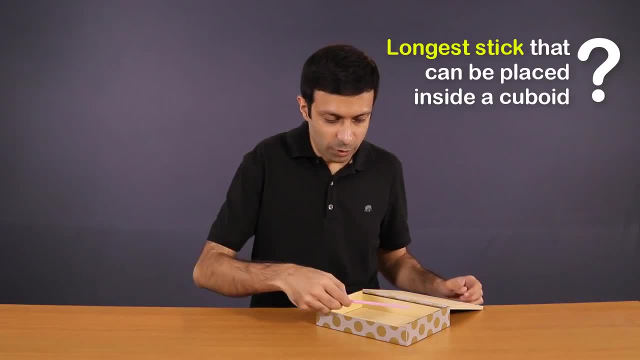 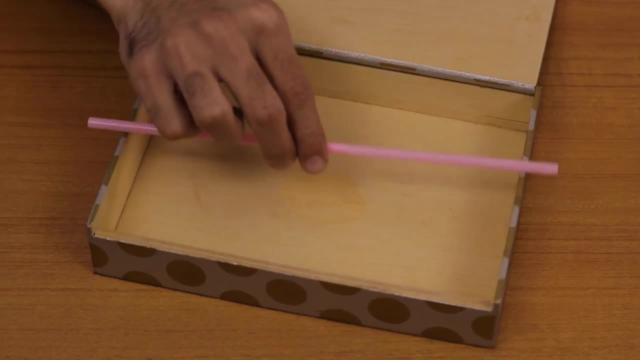 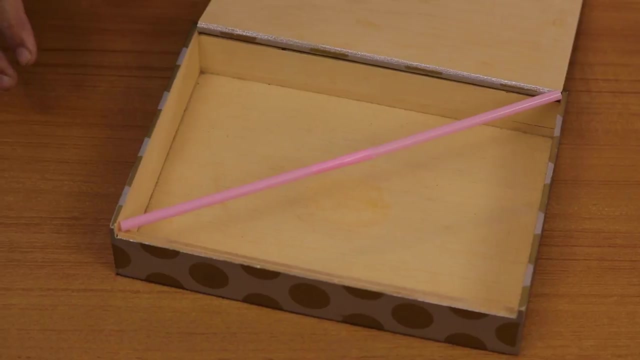 So let's go ahead and try it. Let's try with this stick. So, as you can see, it doesn't fit along the length here, So let's try a different way. If I try to place it like this, again it doesn't fit. This is the. 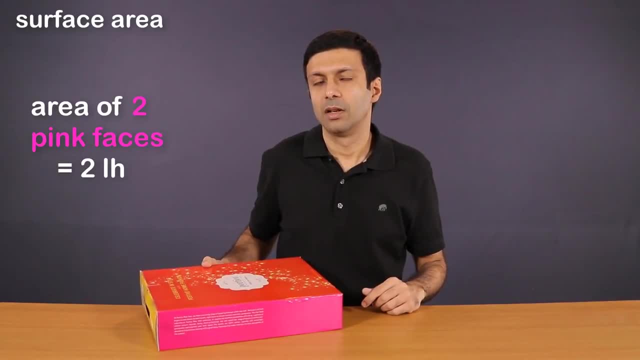 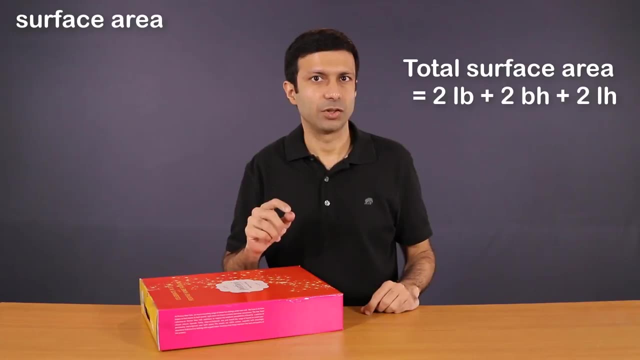 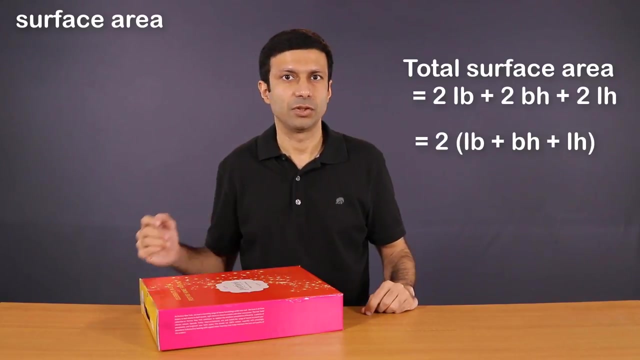 So that's 2LH. So the total surface area is going to be 2LB plus 2BH plus 2LH, So that's 2 into LB plus BH plus LH. There's another term, There's another term called lateral surface area. 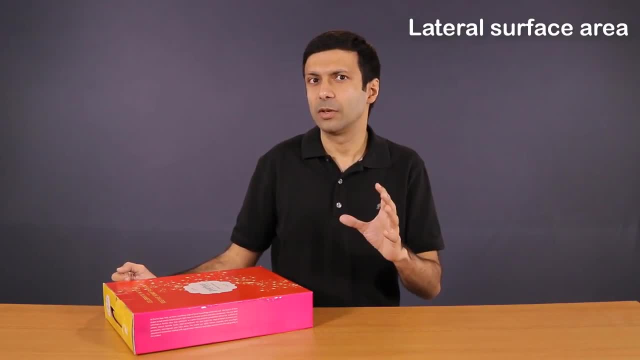 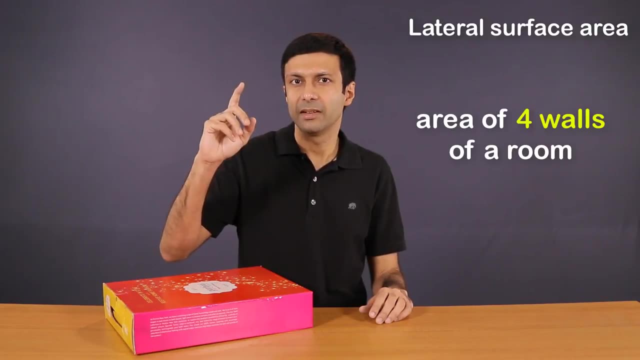 An easy way to remember it is that the lateral surface area is the area of the four walls of your room, So not including the area of the ceiling and of the floor. Now what will be the lateral surface area of the cuboid here? 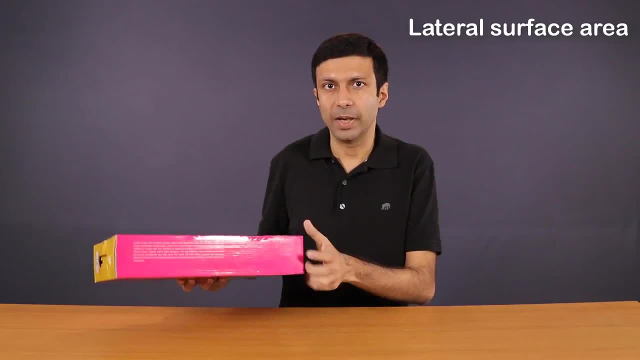 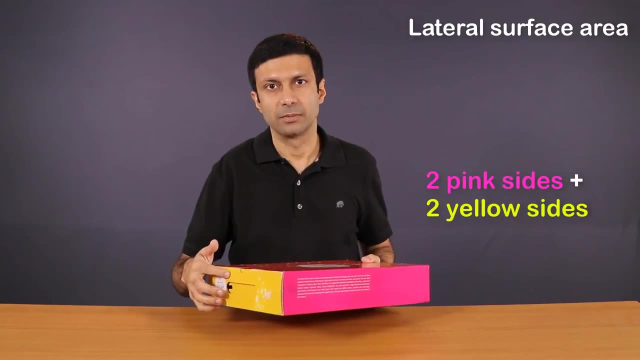 It's going to be the sum of the area of these two pink sides, So these two And the sum of the area of these two yellows And the sum of the area of these two yellow sides. So I'm not including the top and the base here. 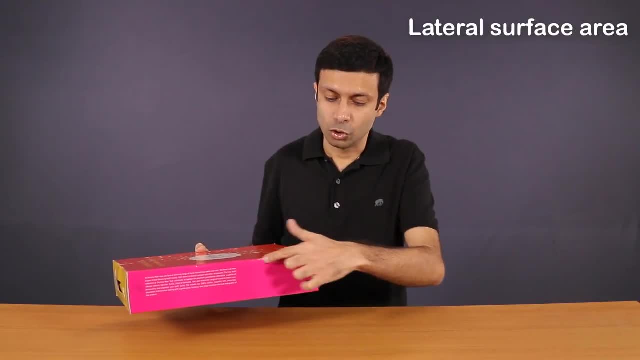 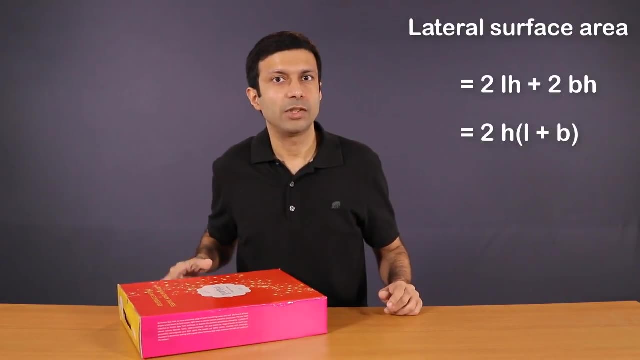 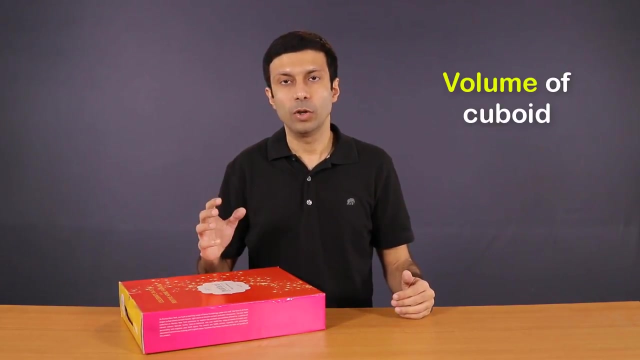 So what will be the formula? It's going to be 2LH plus 2BH, So that's 2H into L plus B. We can also measure the volume of a cuboid. Volume means the space that this box occupies. 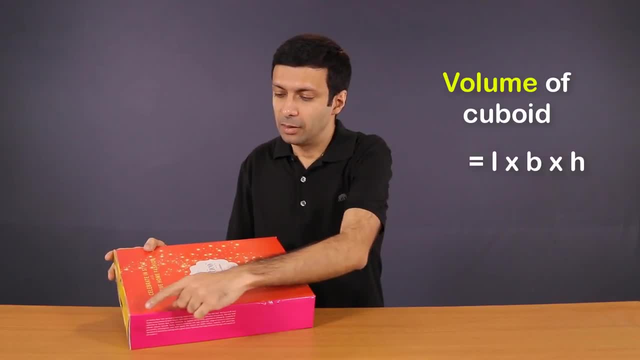 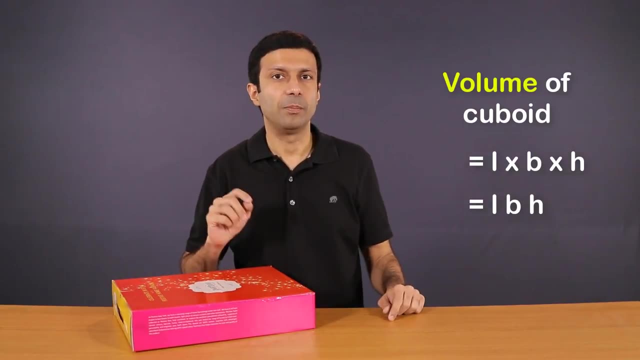 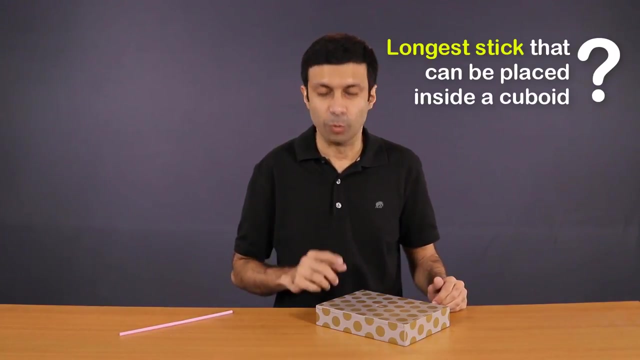 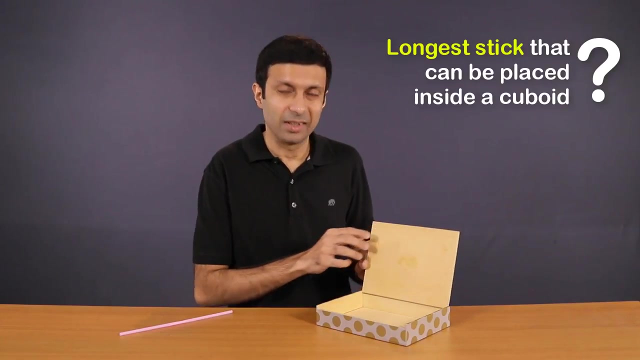 So what is the formula for volume? It's going to be length into breadth, into height, So the formula is LBH. Now an interesting question is: what is the longest stick that we can place inside a cuboid or a box? Here I'm using a different box because it's easy for me to open this one and show you. 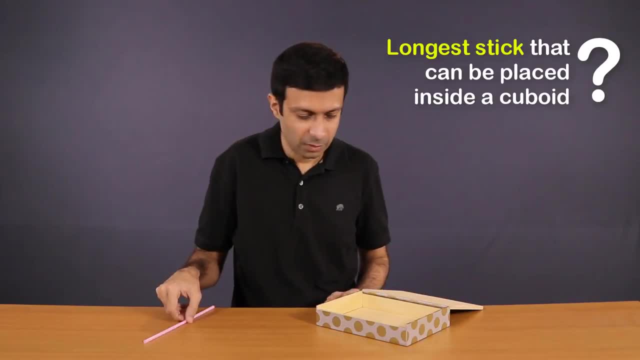 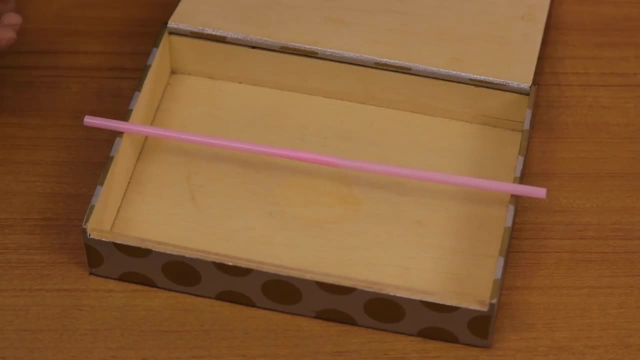 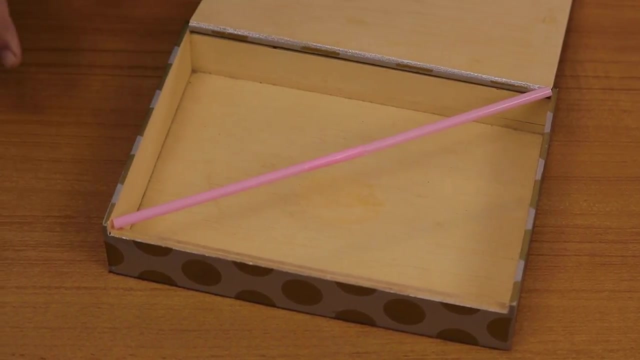 So let's go ahead and try with this stick. So, as you can see, it doesn't fit along the length here, So let's try a different way. If I try to place it like this, again it doesn't fit. This is the diagonal of the rectangle here. 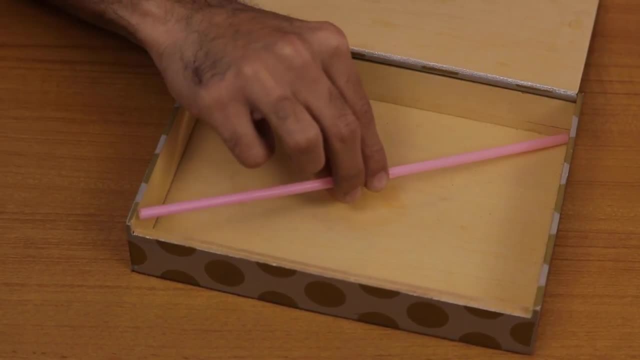 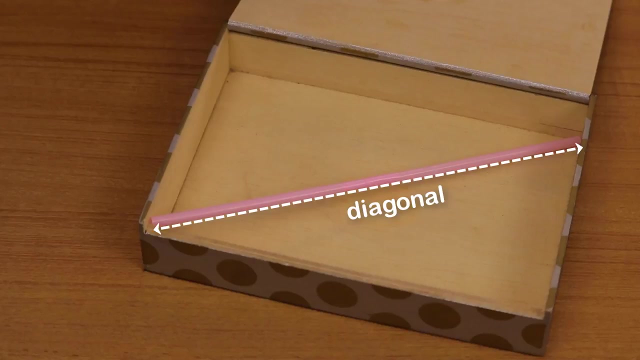 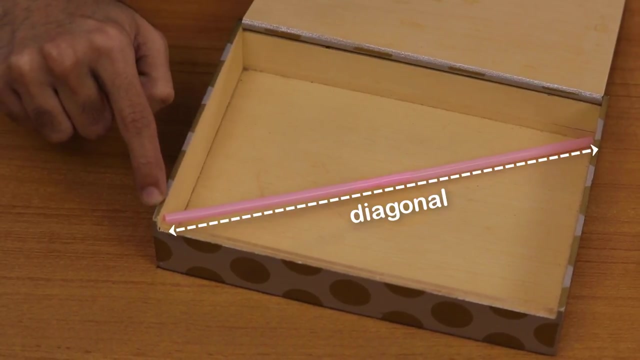 But now, if I place it like this, so as you can see, now it fits in the box. This is the diagonal of the cuboid. This is the longest length inside the box from here to this opposite vertex. here The formula to calculate the length of a diagonal is: 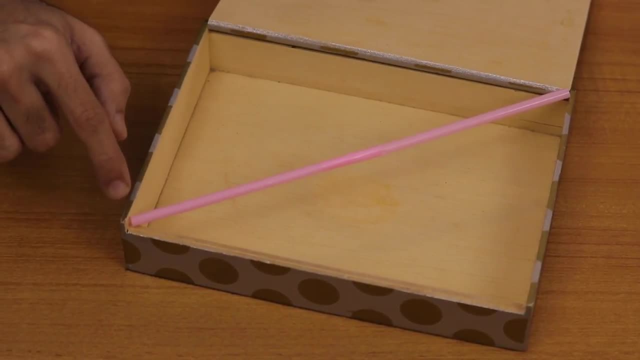 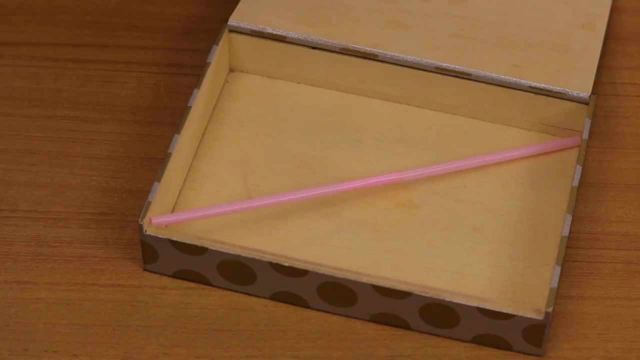 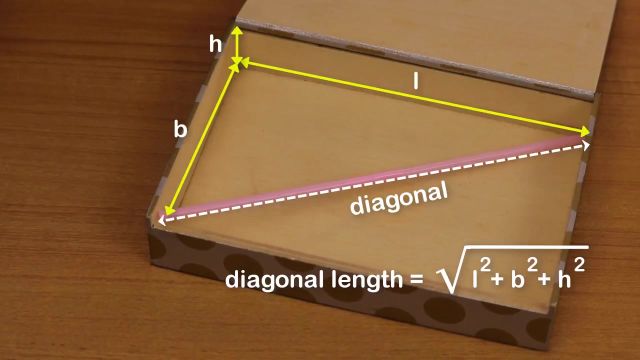 diagonal of the rectangle here. But now, if I place it like this, so as you can see, now it fits in the box, This is the diagonal of the cuboid, the longest length inside the box from here to this opposite vertex. here The formula to calculate the length of a diagonal is square root of L square. 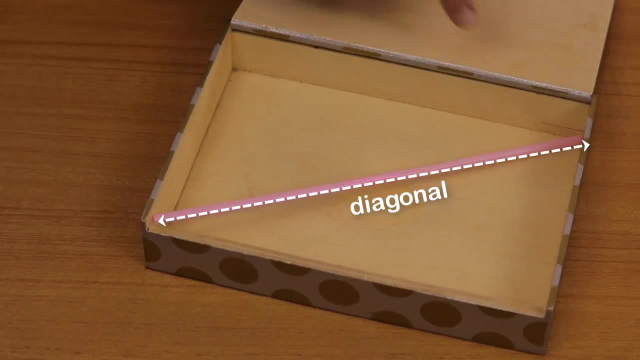 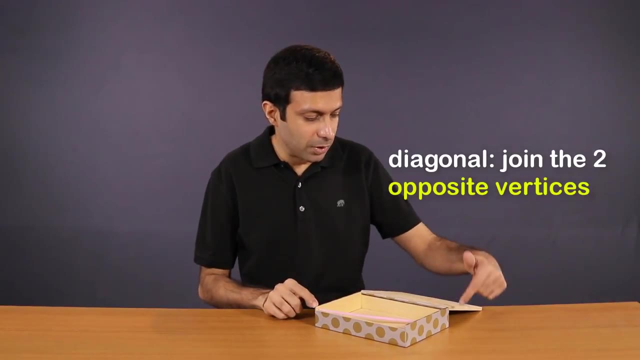 plus B square, plus H square, So that is the longest length that can fit inside a cuboid. So in a diagonal we join the two opposite vertices of a cuboid. So in a diagonal we join the two opposite vertices of a cuboid. 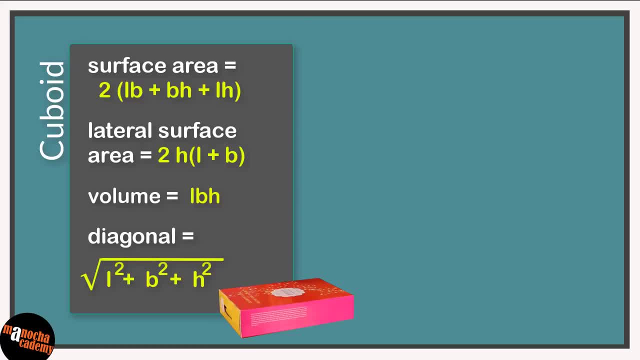 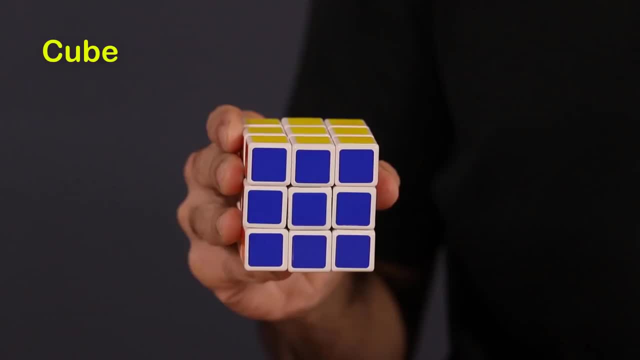 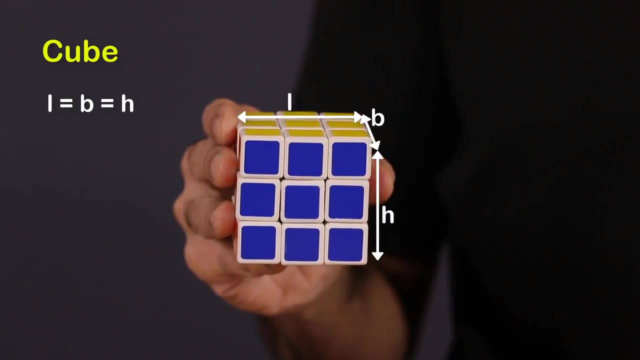 Let's place the formulas that we have learned for a cuboid on our concept board. Now that we are done with the cuboid, let's move on to a cube. A cube is a special cuboid where the length, breadth and height are identical. 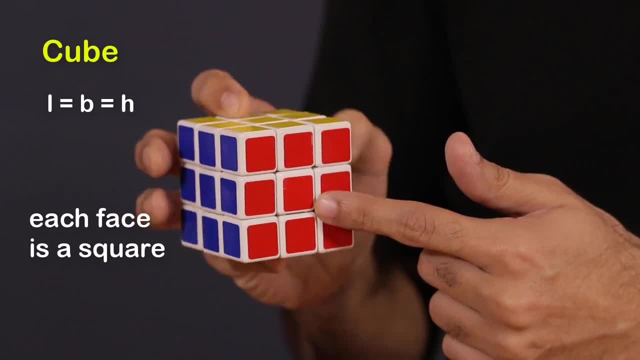 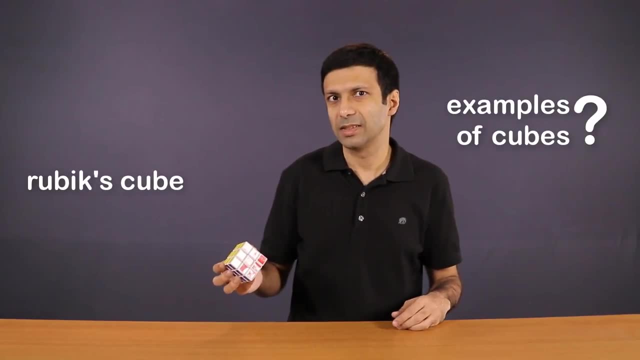 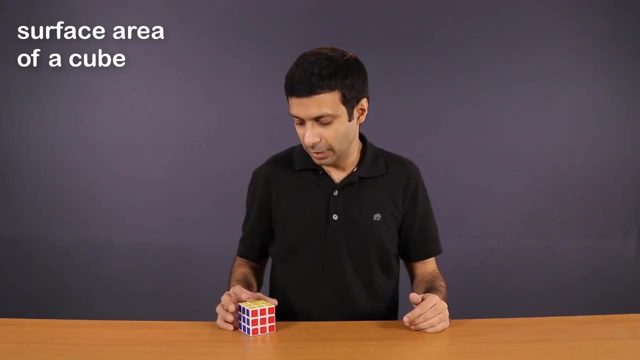 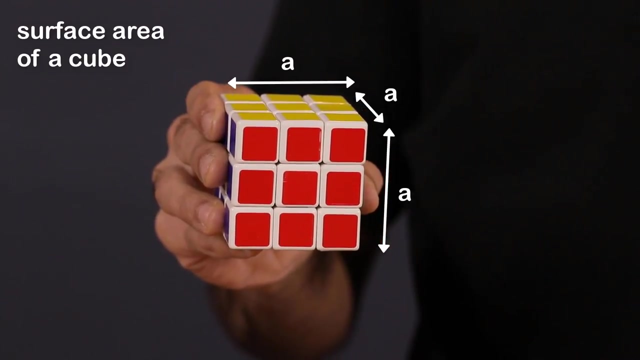 So each face of a cube is a square. Now what are some examples of cubes? One is a row, A Rubik's cube like this. Or another example is a dice. What will be the total surface area of a cube If we represent each side, the length, breadth and height, by the symbol A? then what will? 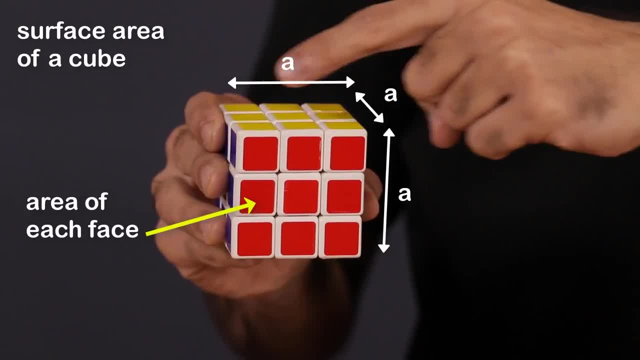 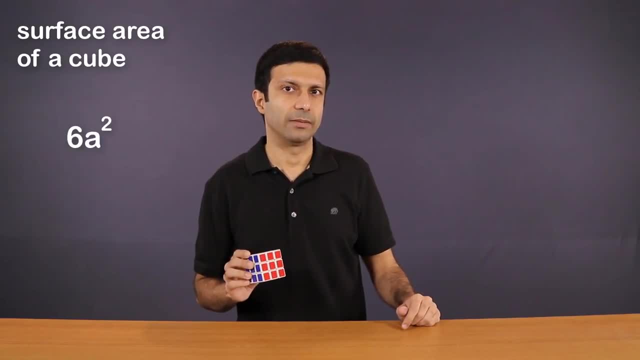 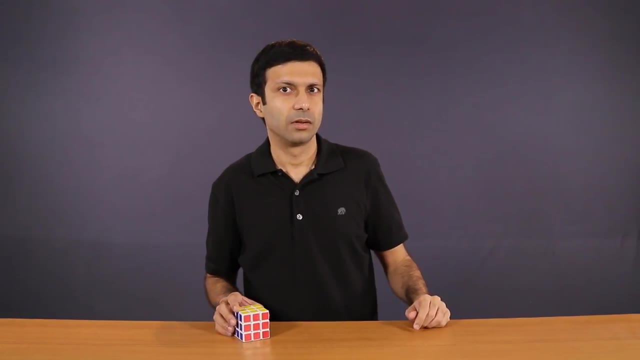 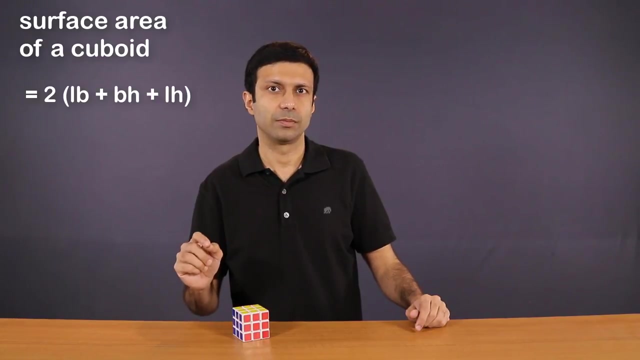 be the area of each face. It's going to be A squared And since there are six faces, the total surface area will be 6A squared. You can also arrive at this formula By using the formula of a cuboid. So the surface area of a cuboid was 2 into LB plus BH plus LH. 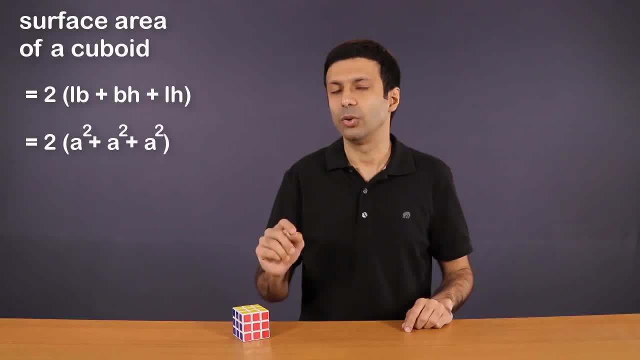 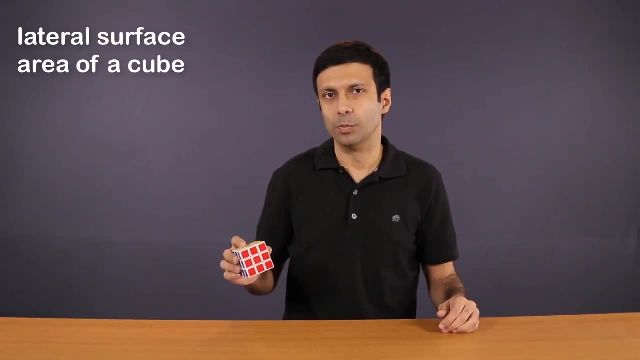 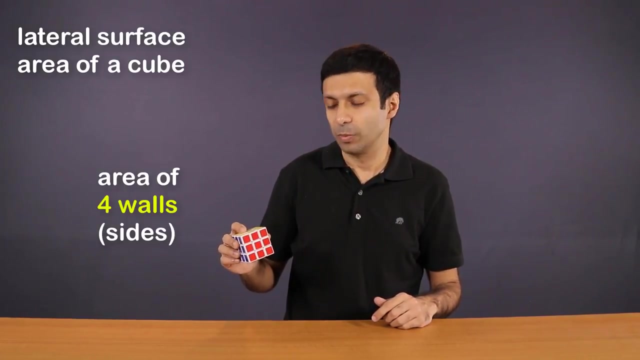 Now, if you substitute LB and H as A, you will get the same formula, 6A, squared. What will be the lateral surface area of a cube? Remember, lateral surface area is the area of the four walls. So the song on A square means the surface area at which the square is the area of the 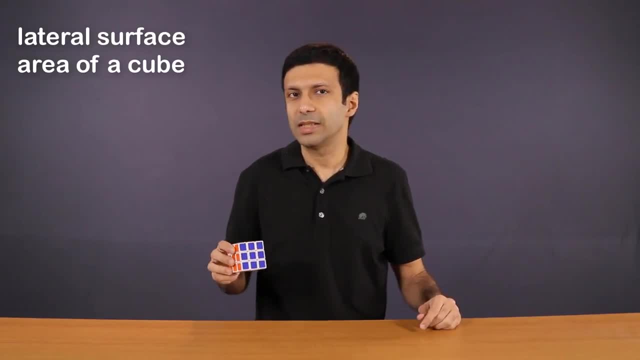 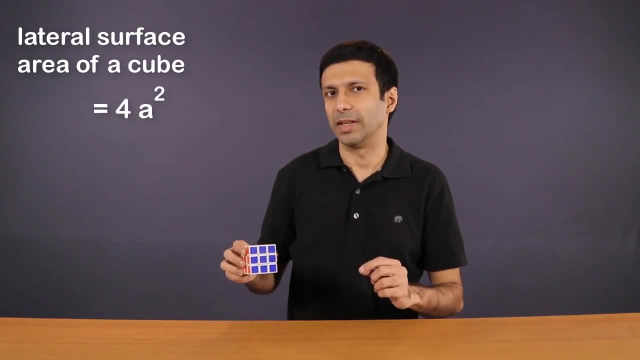 cube itself. You'll think of it as if it's the area of the four sides. What will be the lateral surface area of a cube? It's the area of the four sides. Each side of this area has an area of A squared. 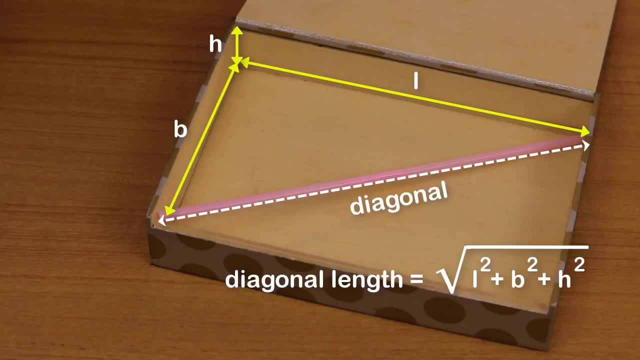 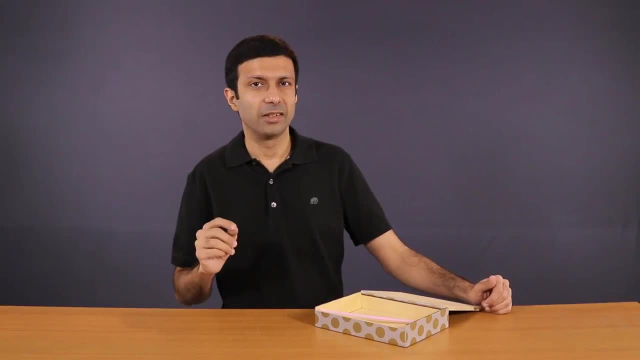 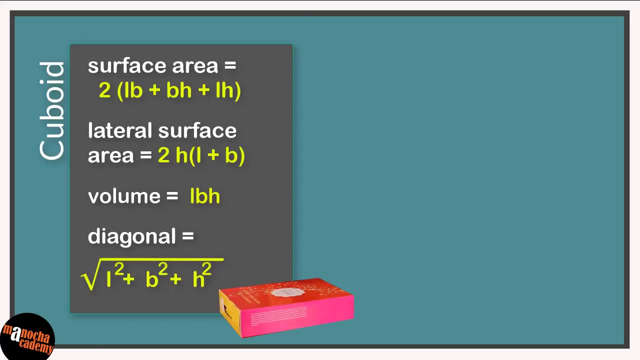 square root of L square plus B square plus H square. So that is the longest length that can fit inside a cuboid. So in a diagonal we join the two opposite vertices of a cuboid. Let's place the formulas that we have learned for a cuboid. 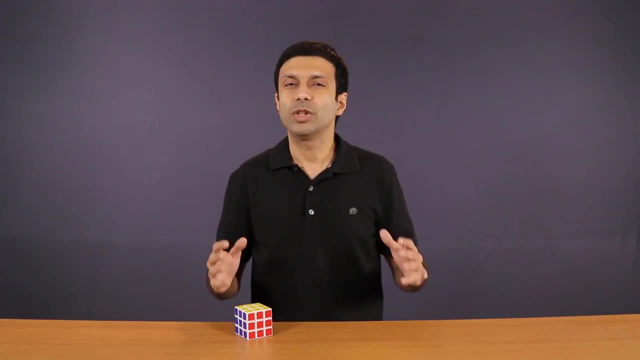 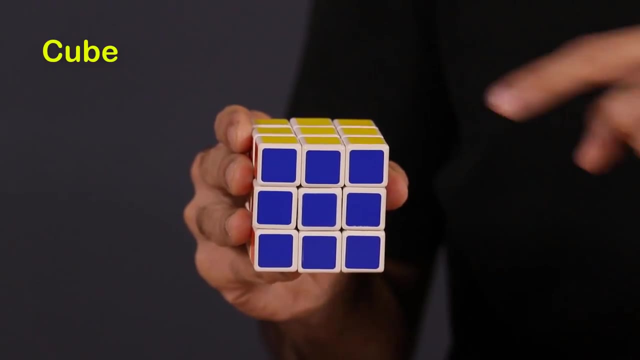 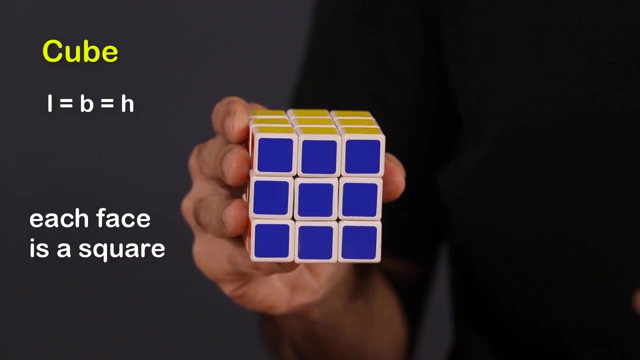 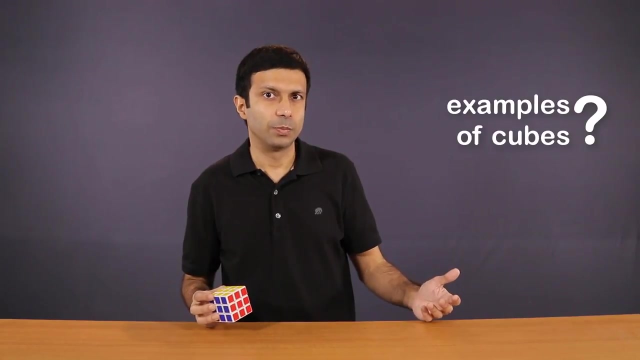 on our concept board. Now that we are done with the cuboid, let's move on to a cube. A cube is a special cuboid where the length, breadth and height are identical, So each face of a cube is a square. Now what are some examples of cubes? 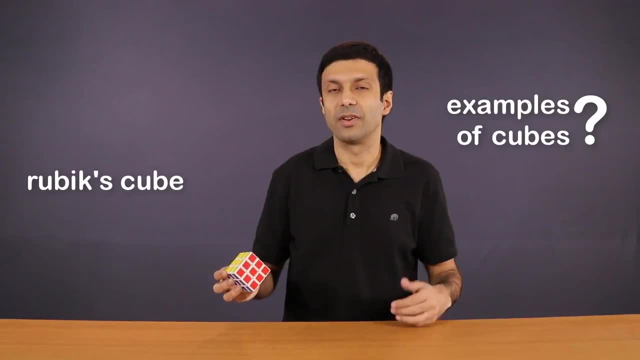 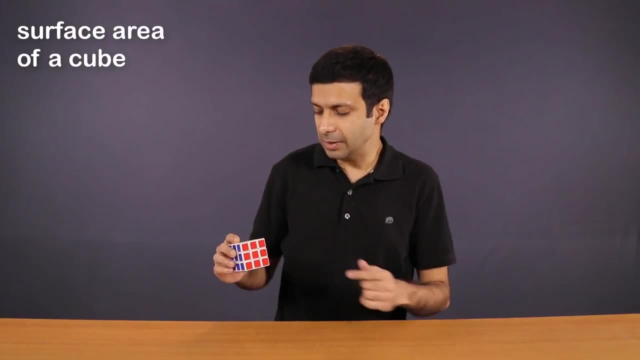 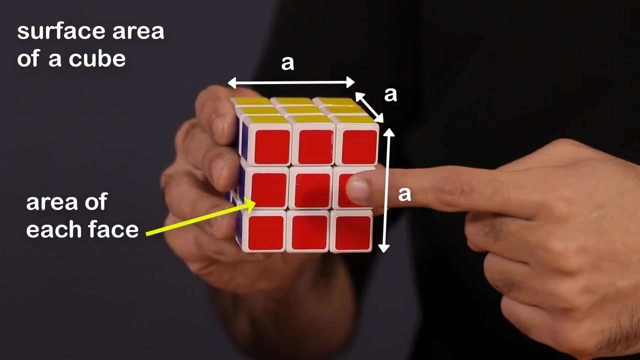 One is a Rubik's cube like this, Or another example is a dice. What will be the total surface area of a cube? If we represent each side, the length, breadth and height by the symbol A, then what will be the area of each face? 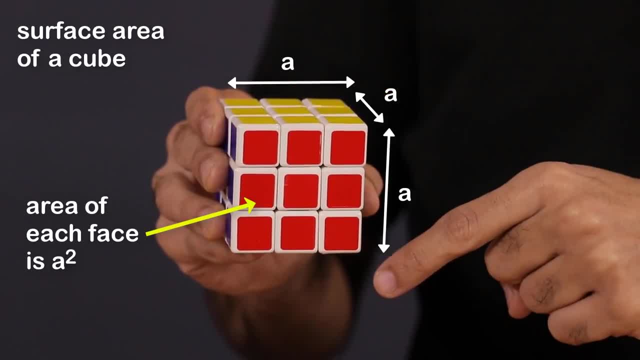 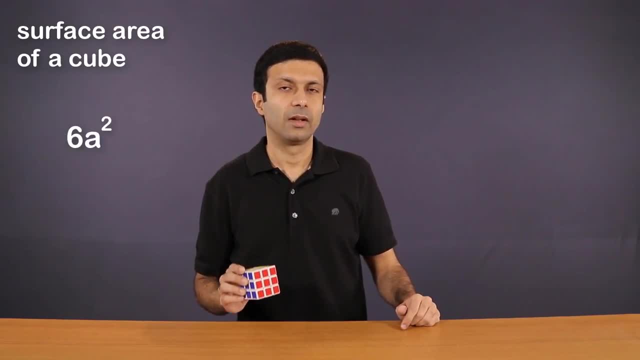 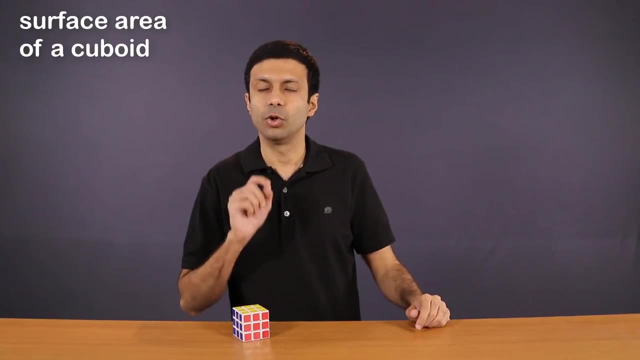 It's going to be A square And since there are six faces, the total surface area will be 6A squared. You can also arrive at this formula by using the formula, which is the formula for a cube. So the surface area of a cuboid was 2 into LB plus BH plus LH. 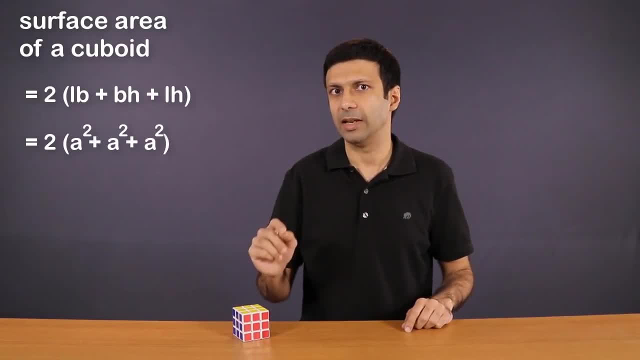 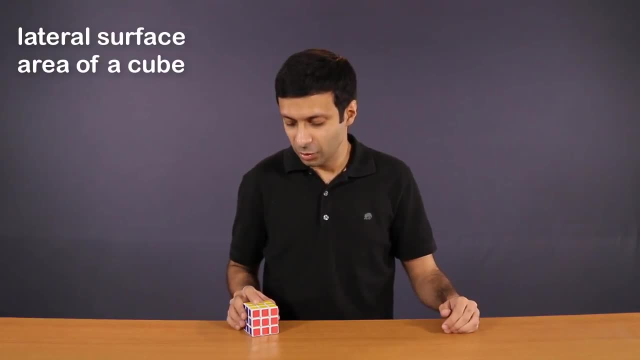 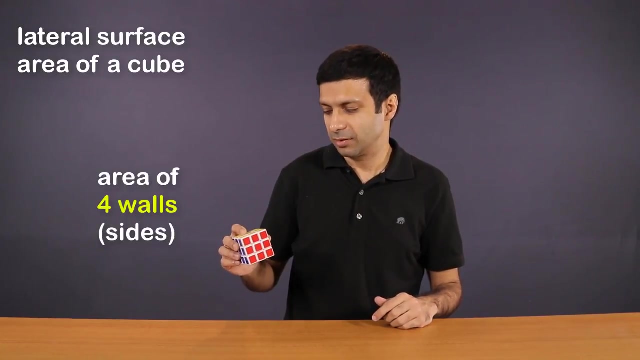 Now, if you substitute LB and H as A, you'll get the same formula, 6A squared. What will be the lateral surface area of a cube? Remember, lateral surface area is the area of the four walls, So it's going to be the area of these four walls. 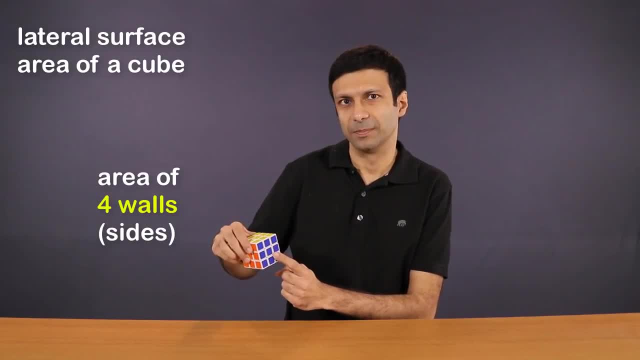 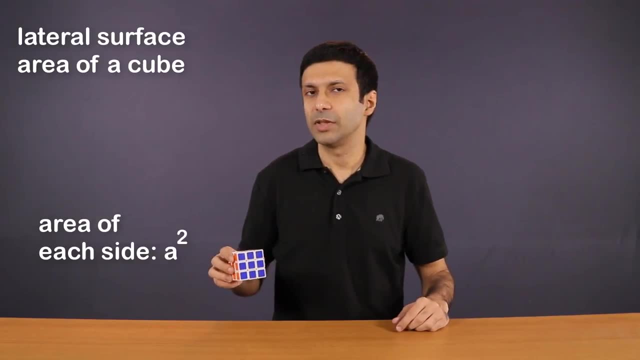 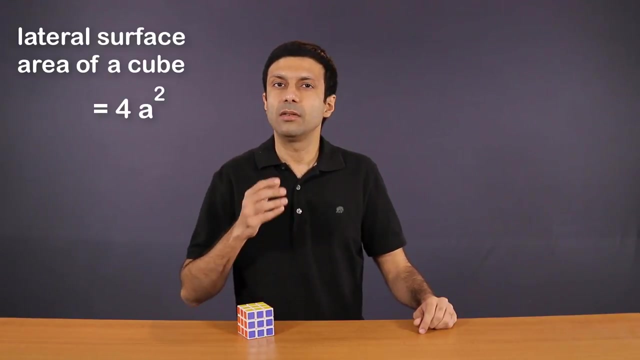 These four sides here And this one Now. each of these sides have an area of A squared, So the lateral surface area will be 4A squared. Again, you can get this formula if you use the formula for lateral surface area of a cuboid. 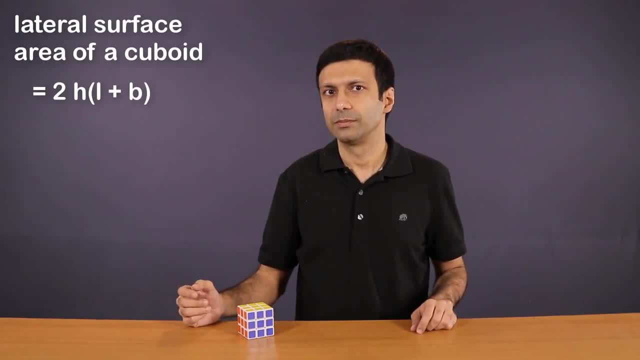 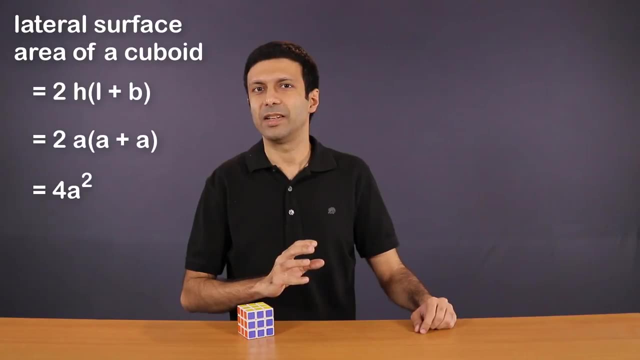 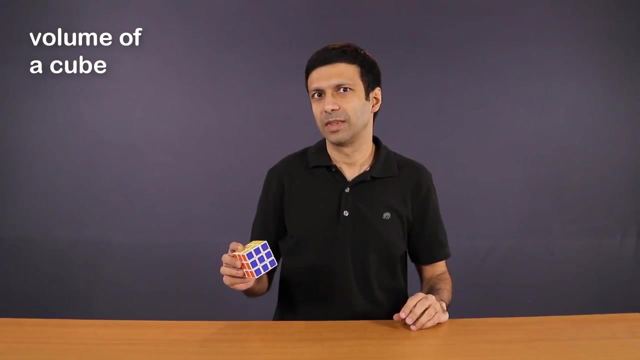 which is 2H, into L plus B. Now, if you substitute LB and H as A, Now if you substitute LB and H as A, you'll get the same formula. Lateral surface area is 4A. squared Volume of a cube is the space it occupies. 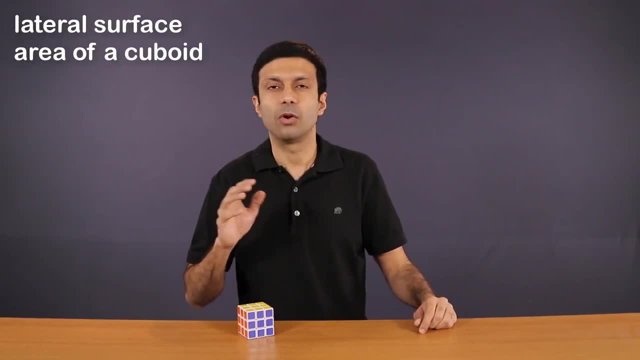 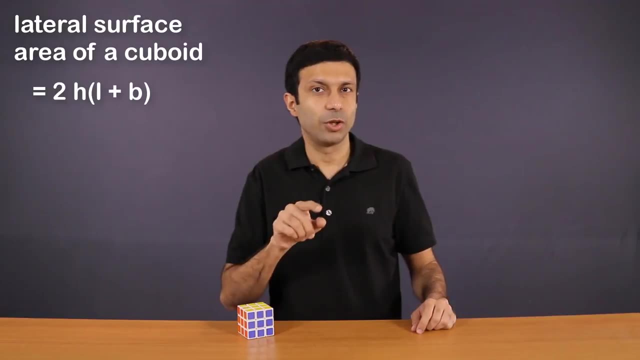 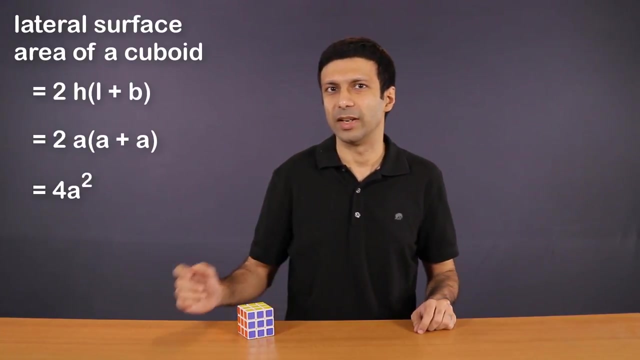 So the lateral surface area will be 4A- squared. Again, you can get this formula if you use the formula for lateral surface area of a cuboid, Which is B and H as A, we'll get the same formula: Lateral surface area is 4A squared Volume. 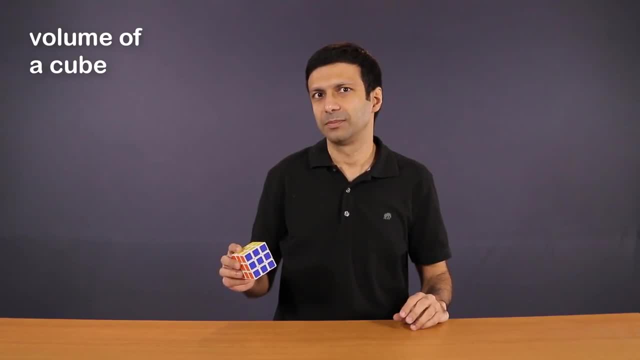 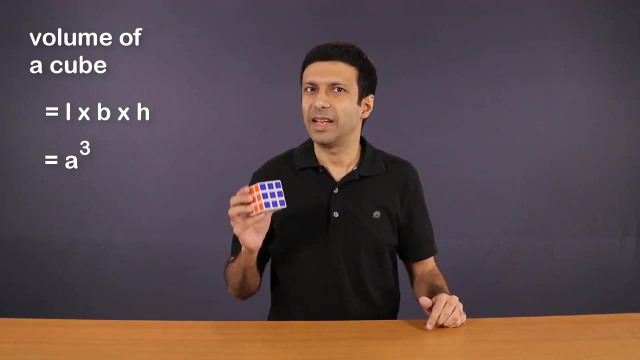 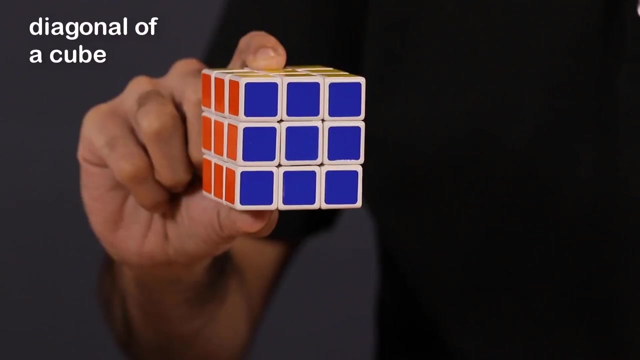 of a cube is the space it occupies, So the volume is going to be L into B, into H, So that's going to be A cube. Diagonal is the longest stick that can be placed inside a cube. So the length of the diagonal is going to be measured from here to here, or you can. 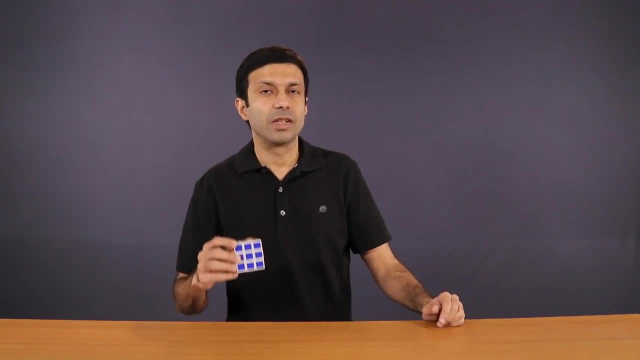 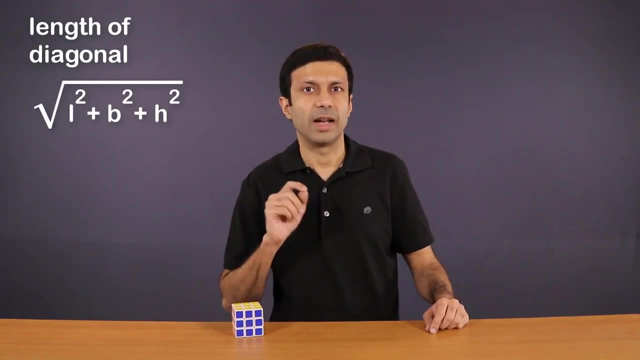 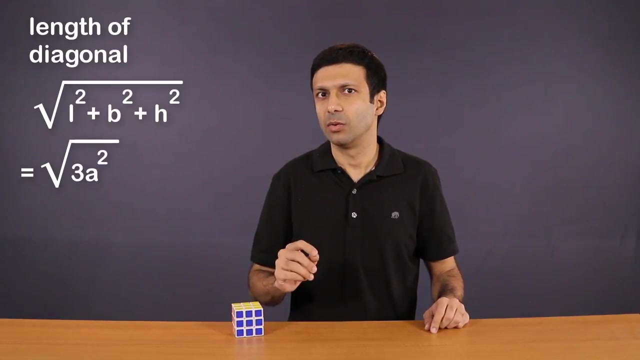 do it from here to here. Now, what is the length of the diagonal? Again, let's use the cuboid formula that we learned, which is square root of L squared plus B squared plus H squared. Now if we substitute L, B and H as A, we get square root of 3A squared. So the length. 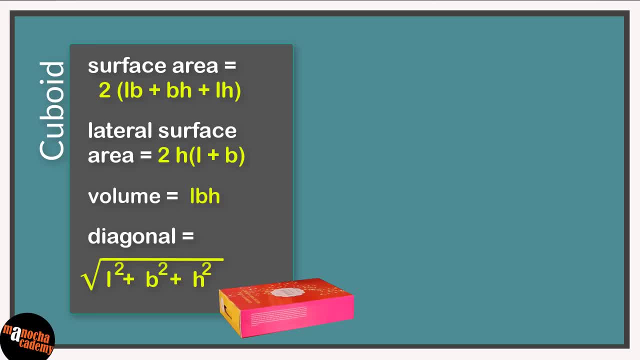 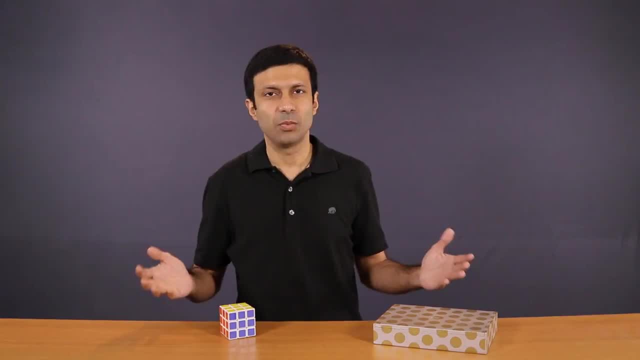 of the diagonal of the cube is going to be L? squared plus B squared plus H squared, The length of the diagonal of a cube is going to be A root 3.. Let's pin the formulas that we learned for a cube on our concept board Now that we are done with the basics of cuboids. 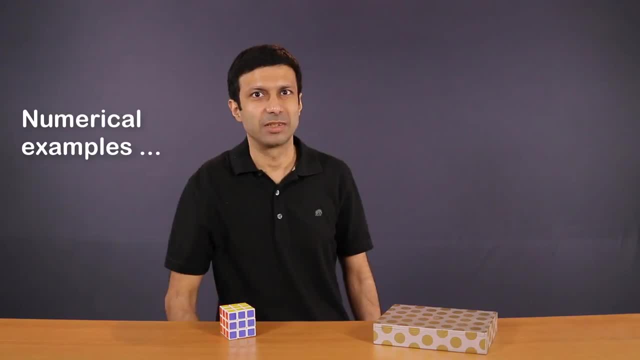 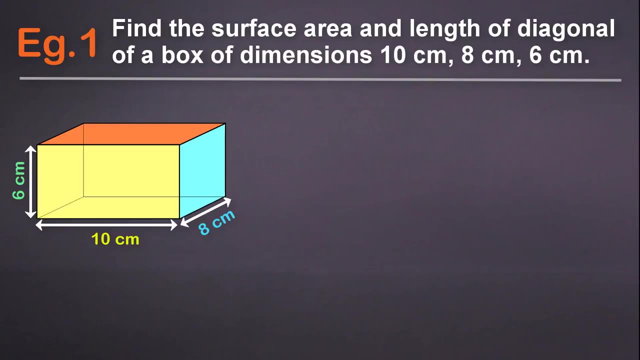 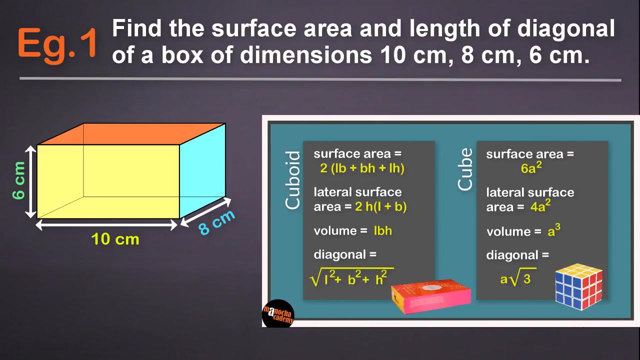 and cubes. let's take a look at some examples. Example 1. Find the surface area and length of the diagonal of a box of dimensions 10 centimeters, 8 centimeters, 6 centimeters. Let's use the surface area and length of the diagonal of a box of dimensions 10 centimeters. 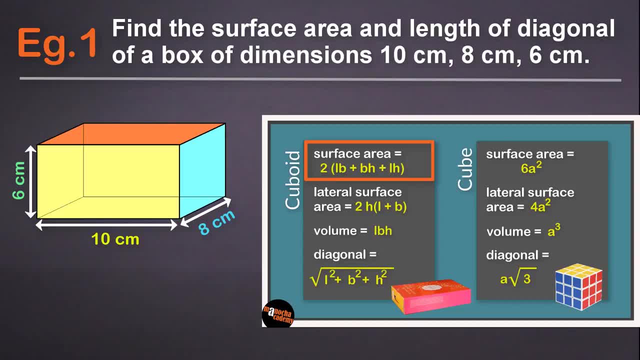 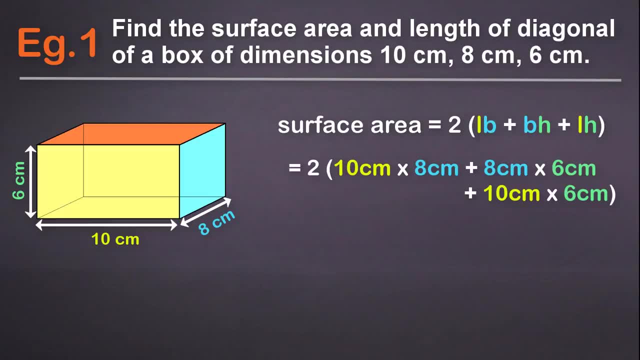 8 centimeters. 8 centimeters. Let's use the surface area formula, which is 2 into LB plus BH plus LH. So substituting the values of L, B and H and calculating, we get 376 centimeters squared. 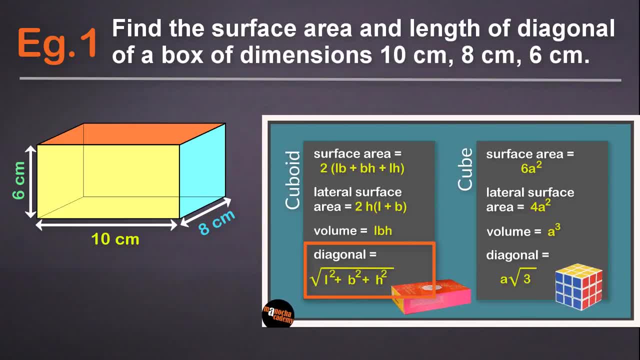 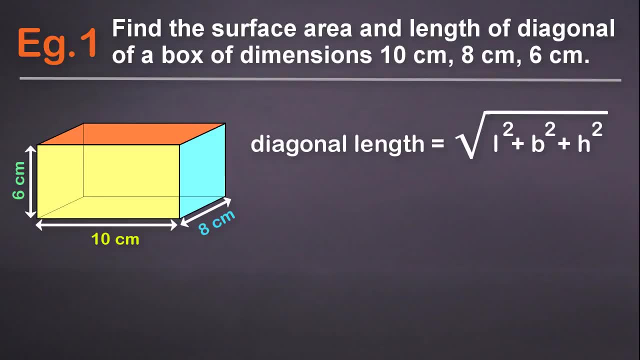 For the diagonal, let's use the diagonal formula, which is square root of L squared plus B squared plus H squared. Plugging in the values, we get 10 root 2 centimeters. So that's the length of our diagonal here. 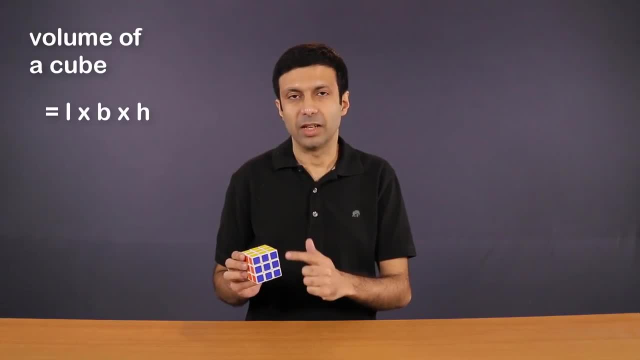 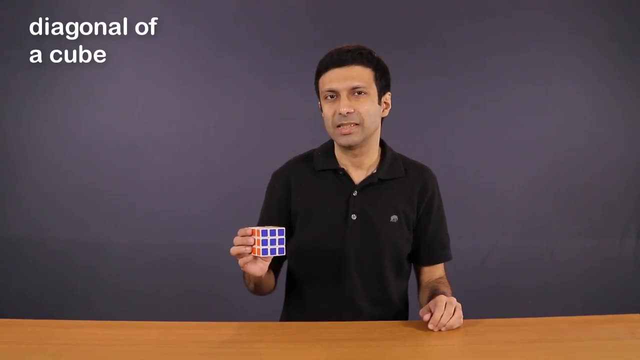 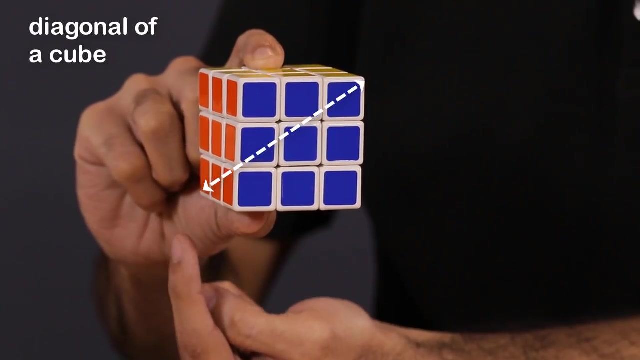 So the volume is going to be L into B, into H. So that's going to be A cubed Diagonal is the longest stick that can be placed inside a cube, So the length of the diagonal is going to be measured from here to here. 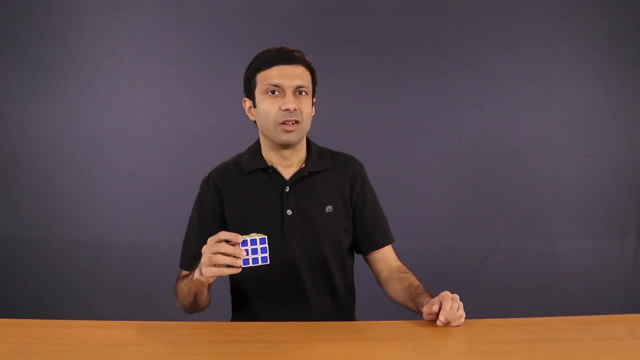 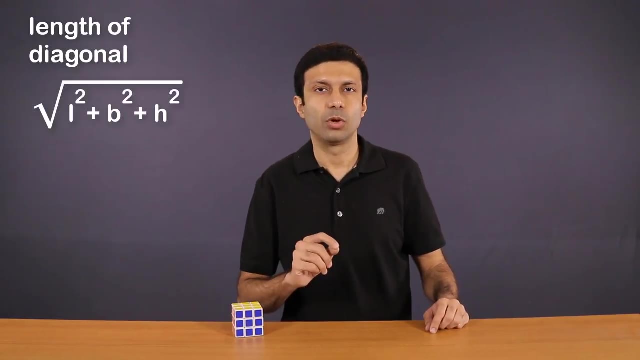 Or you can do it from here to here. Now, what is the length of the diagonal? Again, let's use the cuboid formula that we learned, which is square root of L squared plus B squared plus H squared. Now, if you substitute LB and H as A, 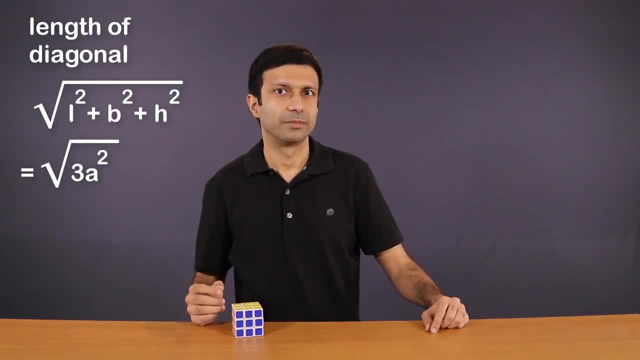 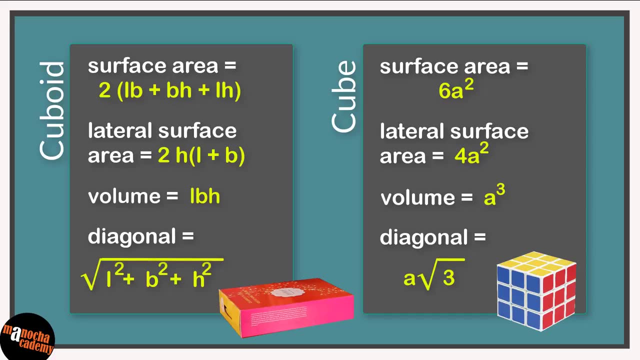 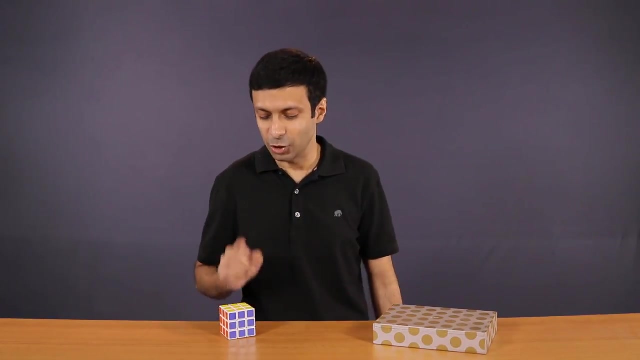 we get square root of 3A squared, So the length of the diagonal of a cube is going to be A root 3.. Let's pin the formulas that we learned for a cube on our concept board, Now that we are done with the basics of cuboids and cubes. 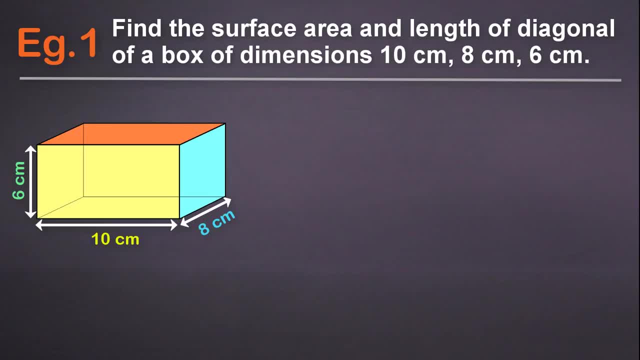 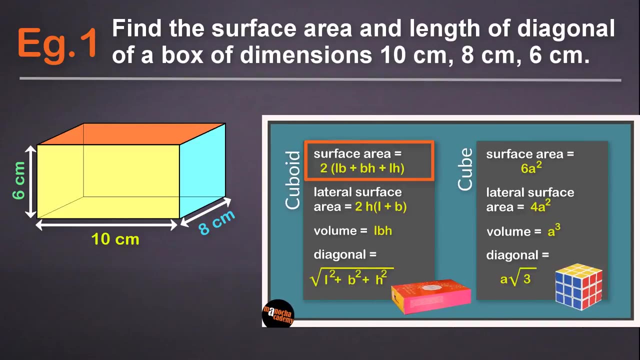 let's take a look at some examples. Example 1. Find the surface area and length of the diagonal of a box of dimensions 10 centimeters, 8 centimeters, 6 centimeters. Let's use the surface area formula, which is 2 into LB. 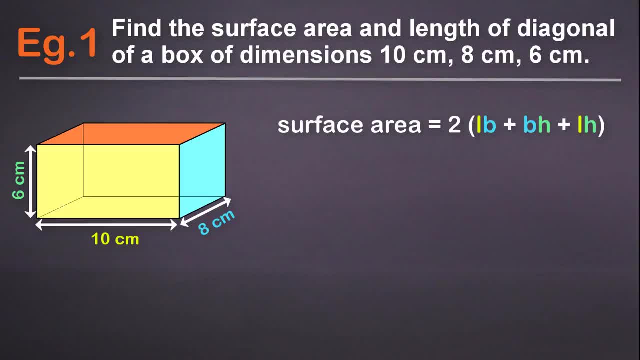 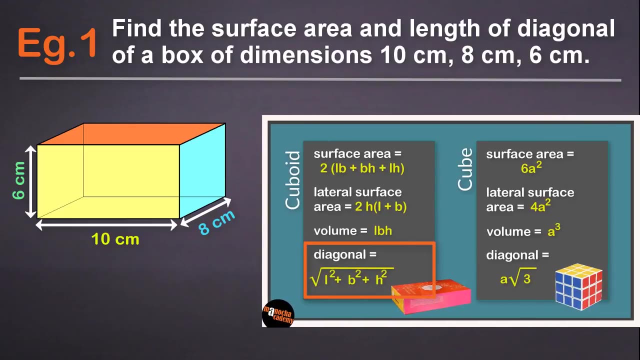 plus BH plus LH. So substituting the values of LB and H and calculating, we get 376 centimeters squared. For the diagonal, let's use the diagonal formula which is square root of L squared plus B squared plus H squared. 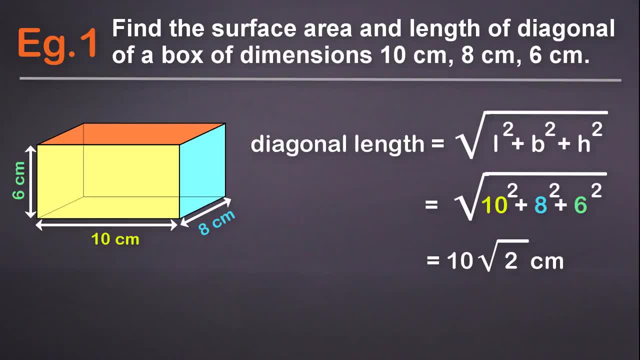 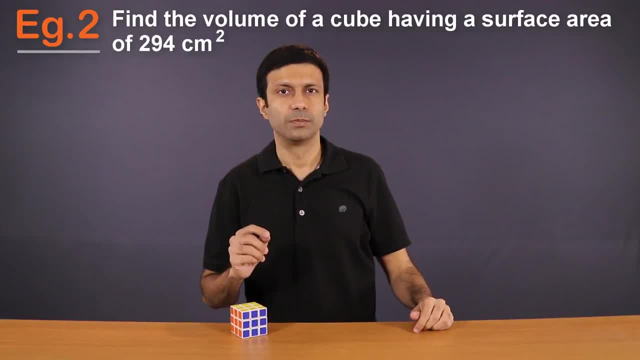 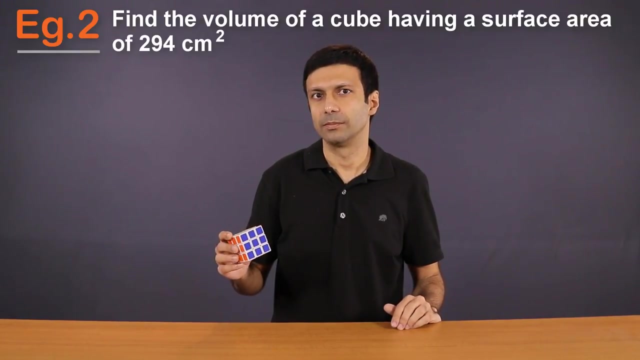 Plugging in the values we get 10 root 2 centimeters. So that's the length of our diagonal here. Example 2.. Find the volume of a cube having a surface area of 294 centimeters squared. Let's say our Rubik's cube here has a surface area of 294 centimeters squared. 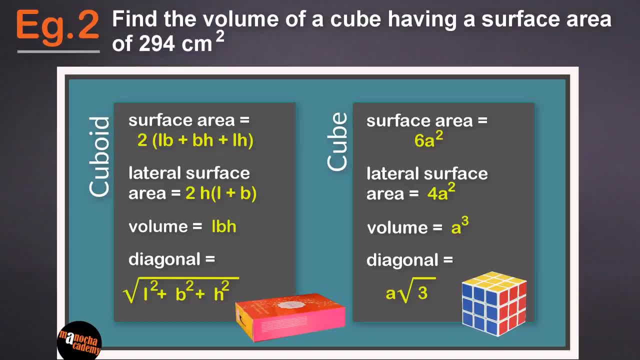 Now, how do we find its volume? So, looking up our formula list, to find the volume of this cube we actually need the side which is represented by A, So let's use the surface area formula. So we have: 6A squared equals 294.. 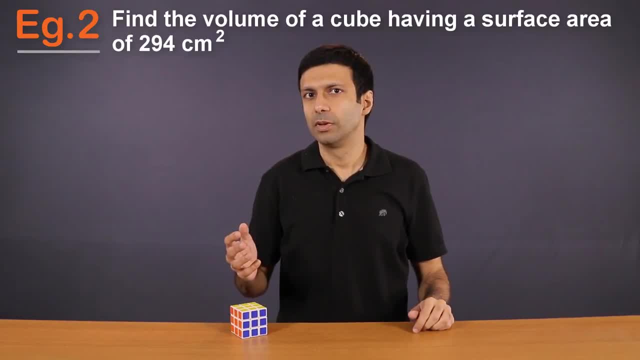 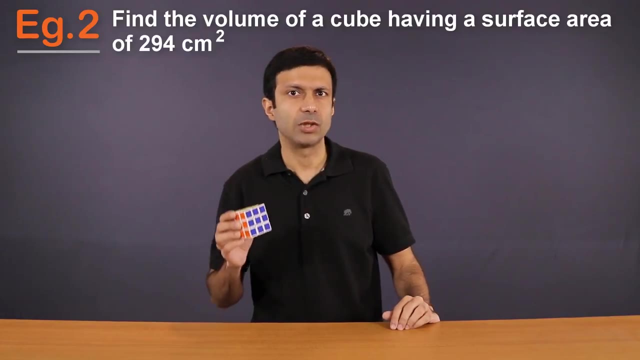 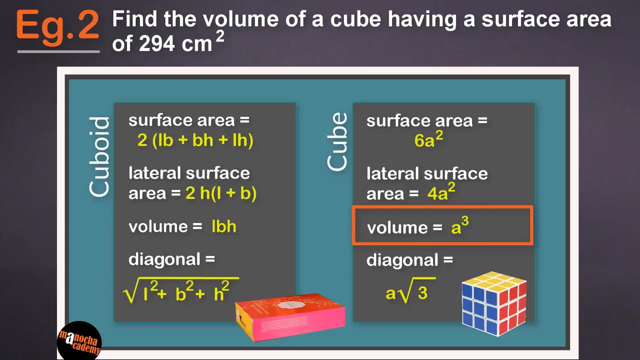 Example 2.. Find the volume of a cube having a surface area of 294 centimeters squared. Let's say our Rubik's cube here has a surface area of 294 centimeters squared. Now how do we find its volume? So, looking up our formula list, to find the volume of this cube we actually need the side which is represented by A. 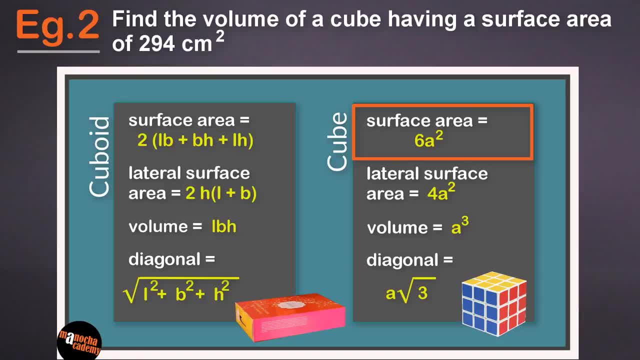 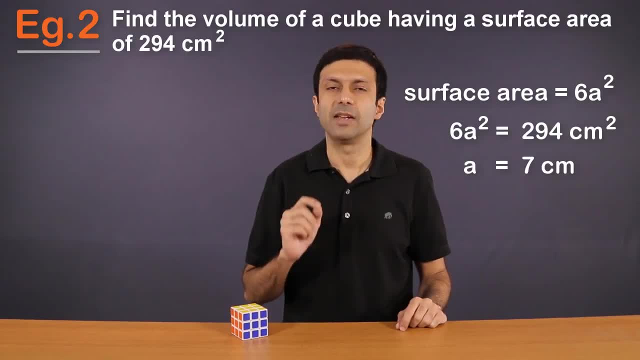 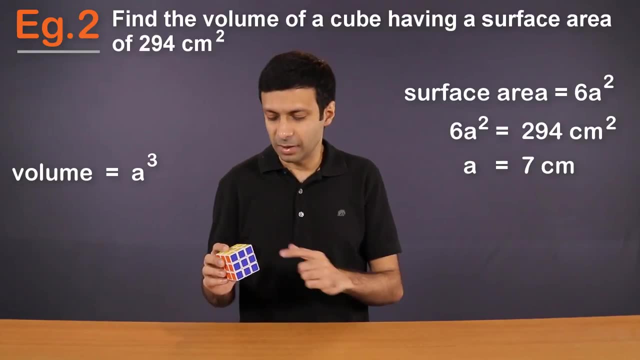 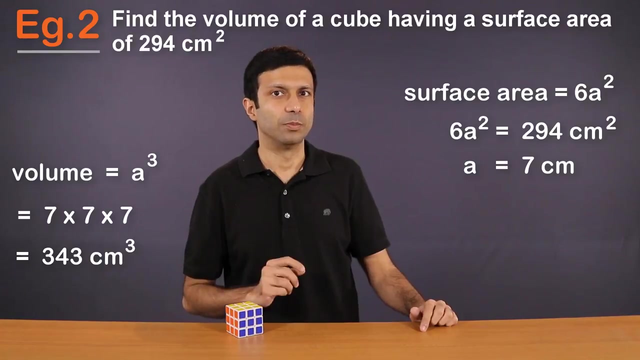 So let's use the surface area formula. So we have: 6A squared equals 294.. And solving, we get A as 7 centimeter. So the volume of this cube is going to be A cube which is 7.. Into 7, into 7,, so that's 343 centimeter cube. 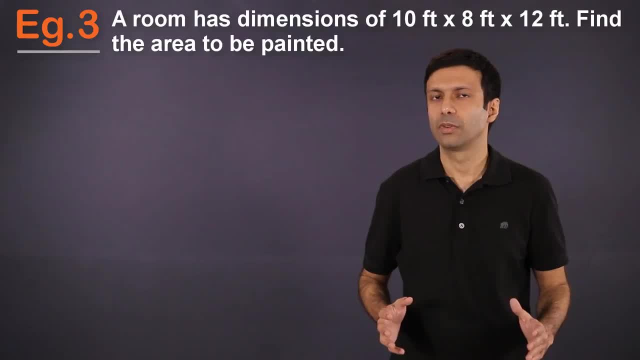 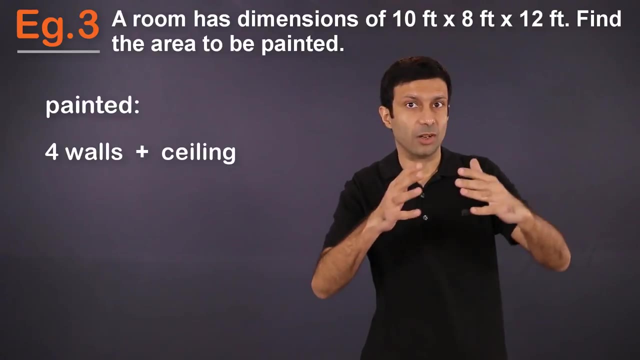 Example 3.. A room has a dimensions of 10 feet by 8 feet by 12 feet. Find the area to be painted. So if you look around in the room that you're in, what needs to be painted It's the walls around you and the ceiling. 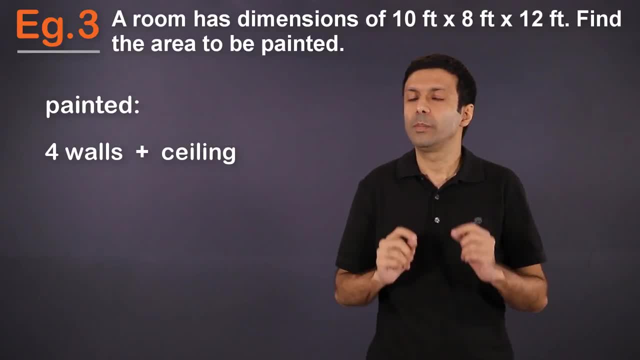 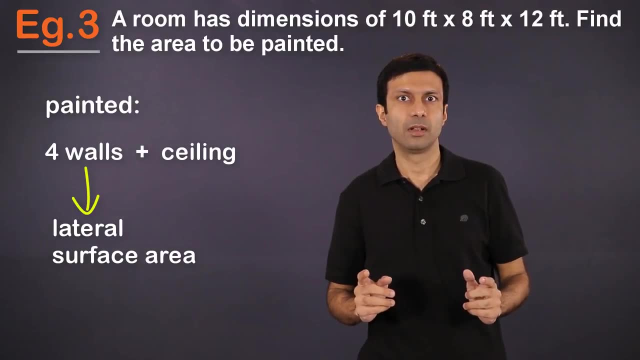 We don't need to paint the floor. So what will be the total area? It's going to be the area of the walls, So that's the lateral surface area plus the area of the ceiling. So what are the formulas we'll use? 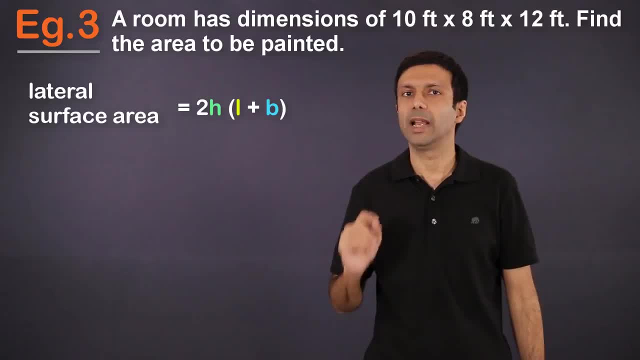 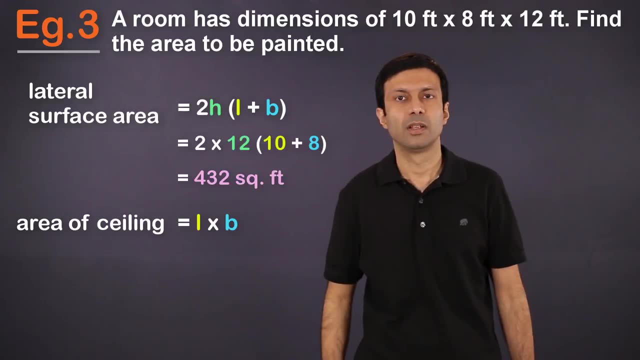 Lateral surface area is 2H into L plus B And the area of the ceiling is going to be length into the breadth. So if we add up all the numbers we're going to get a total area of 512 square feet. 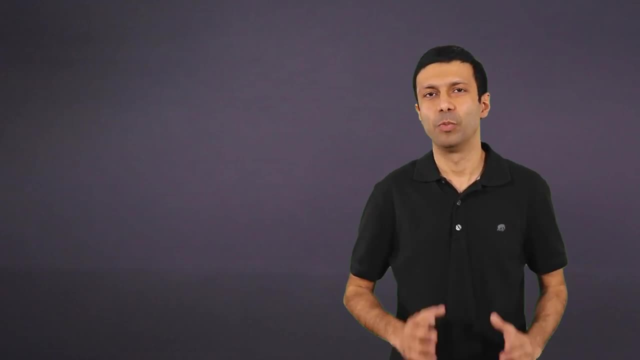 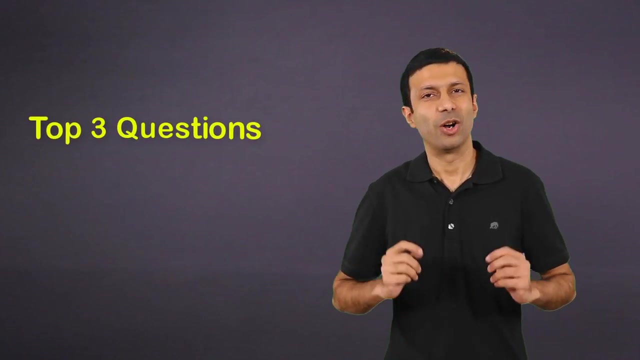 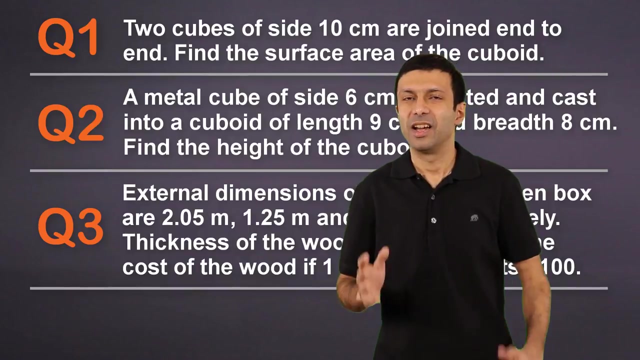 I hope now you have an idea how to solve the sums of cuboids and cubes. So let's move on to our top three test-oriented questions on this topic Coming up for you. I would like you to pause here and try to solve these questions. 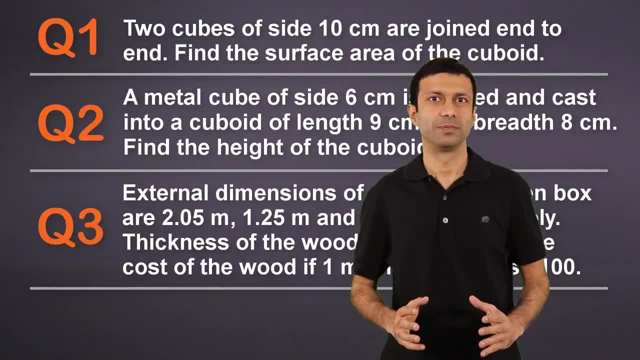 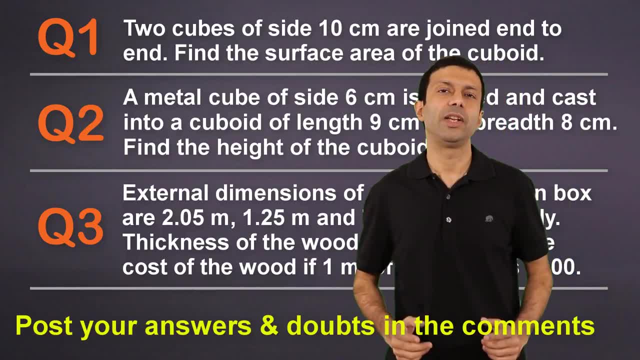 Let's make this more interactive than just watching the video. So do post your answers In the comments below, Or, if you have any doubts, feel free to write it in the comments below, And I promise to answer all of them promptly. So I'm going to move off and let you solve these questions. 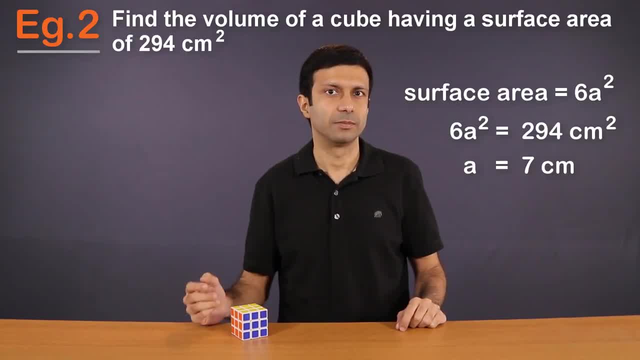 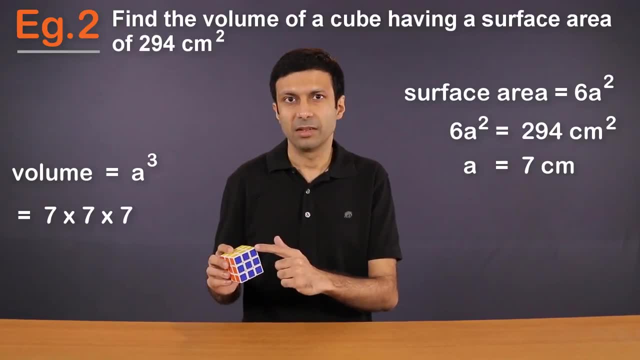 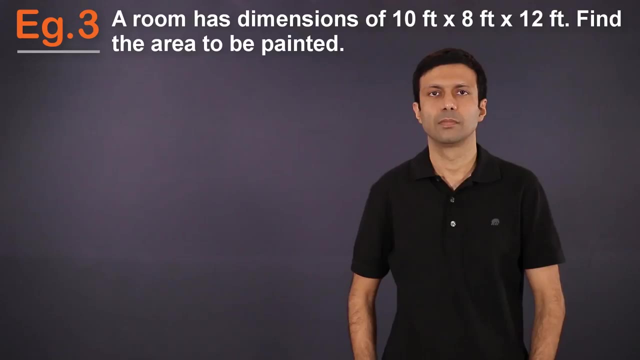 And solving, we get A as 7 centimeter. So the volume of this cube is going to be A cube which is 7 into 7 into 7.. So that's 343 centimeters squared. Example 3.. A room has a dimensions of 10 feet by 8 feet by 12 feet. 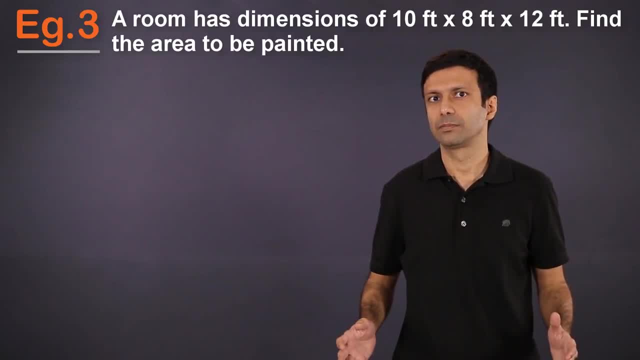 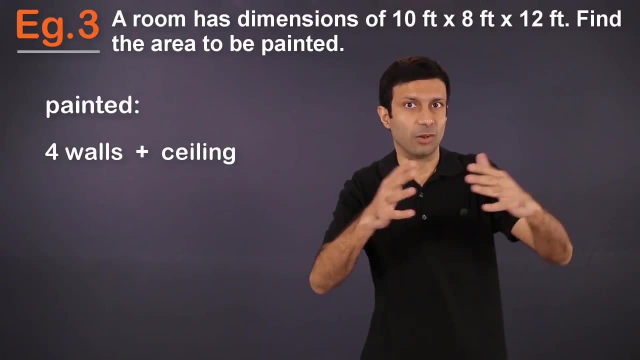 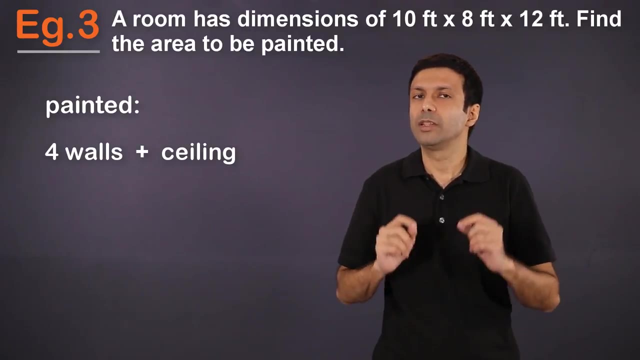 Find the area to be painted. So if you look around in the room that you're in, what needs to be painted It's the walls around you and the ceiling. We don't need to paint the floor right. So what will be the total area? 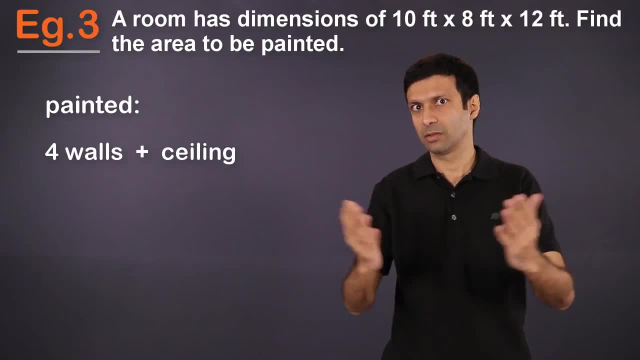 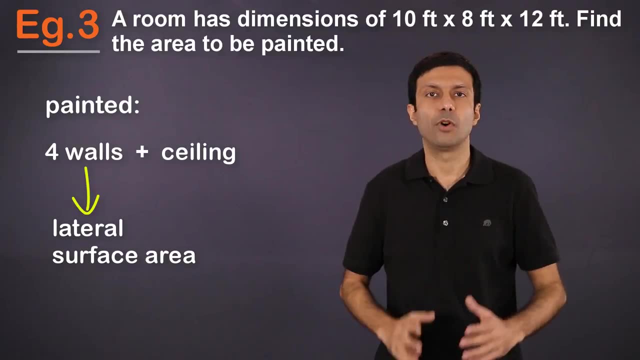 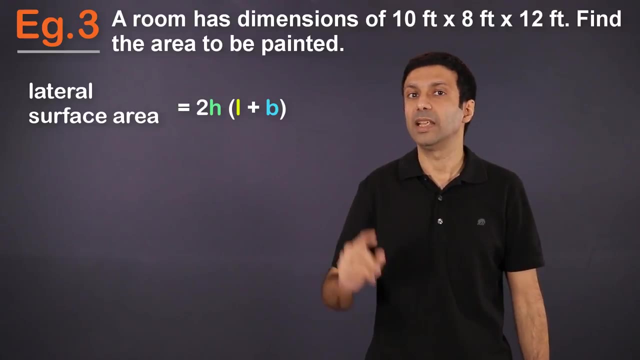 It's going to be the area of the walls, So that's the lateral surface area plus the area of the ceiling. So what are the formulas we'll use? Lateral surface area is 2H into L plus B And the area of the ceiling is going to be length into the breadth. 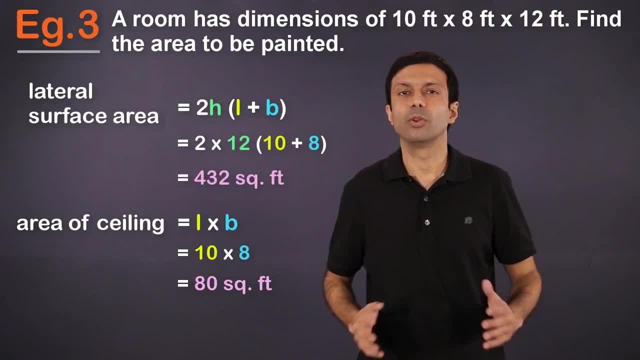 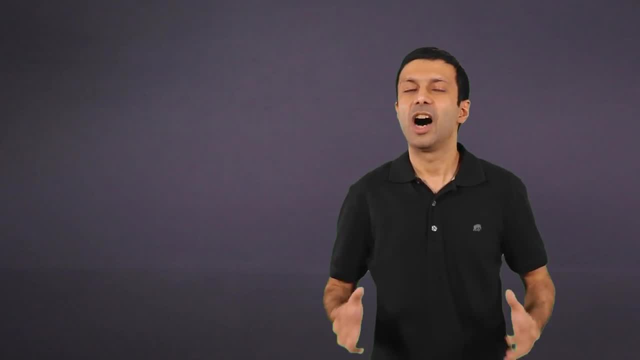 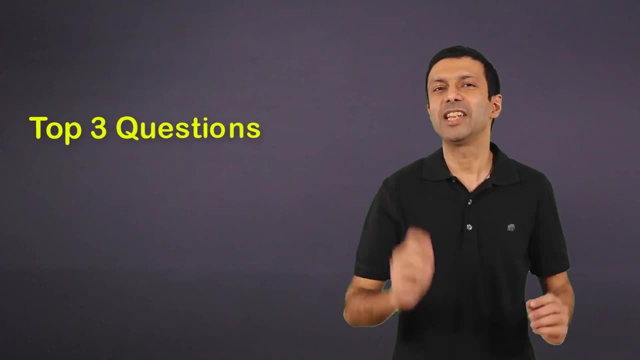 So if we add up all the numbers, we're going to get a total area of 512 square feet. I hope now you have an idea how to solve the sums of cuboids and cubes. So let's move on to our top three test-oriented questions on this topic. 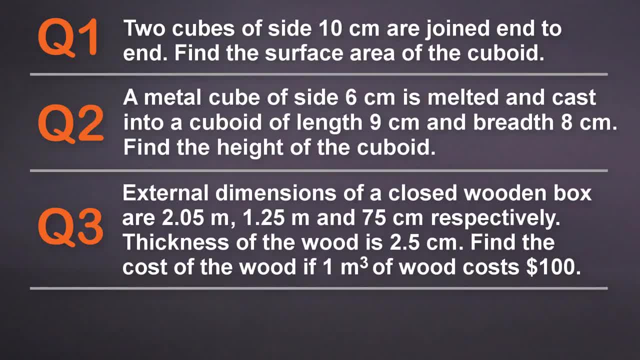 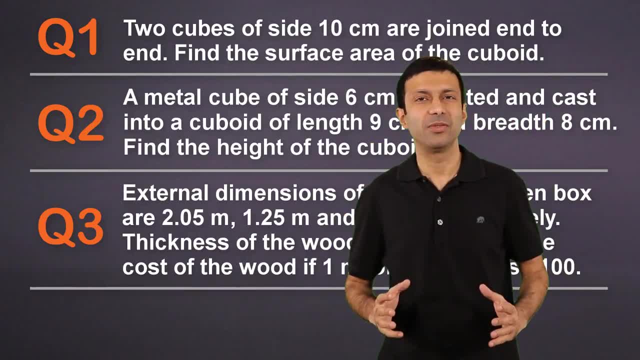 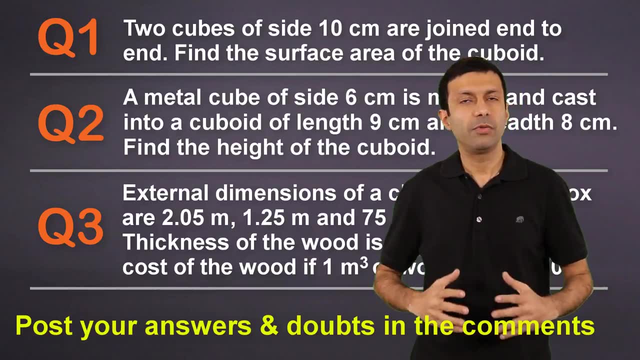 Coming up for you. I would like you to pause here and try to solve these questions. Let's make this more interactive than just watching the video. So do post your answers in the comments below Or, if you have any doubts, feel free to write it in the comments below. 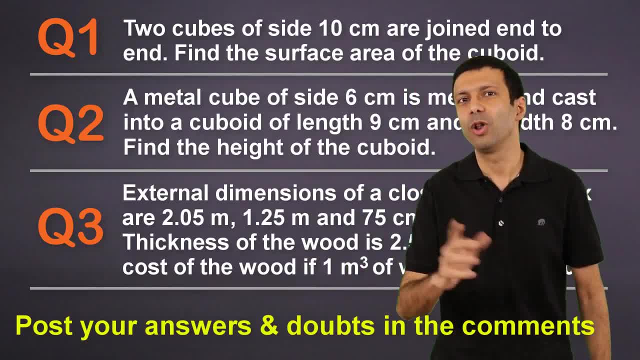 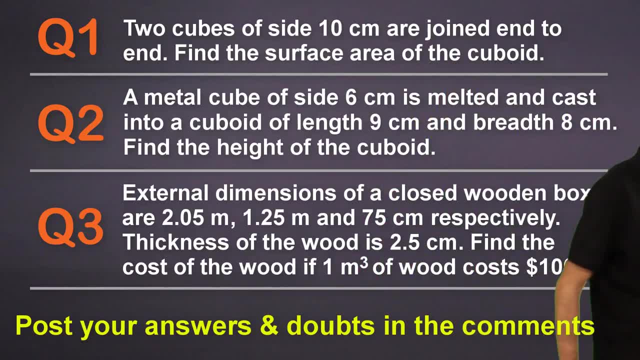 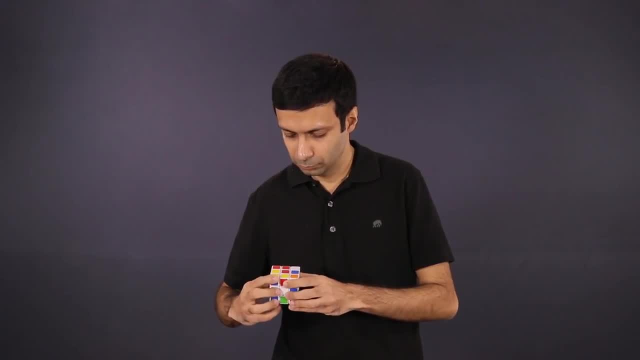 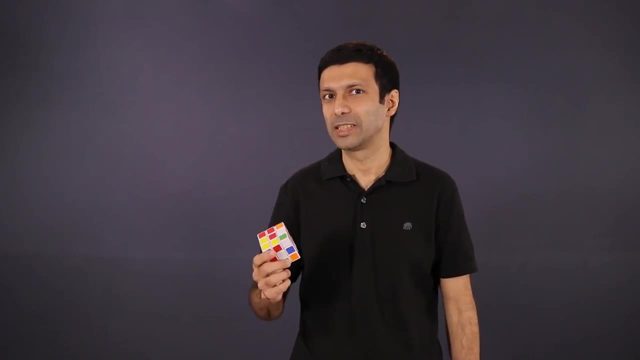 And I promise to answer all of them promptly. So I'm going to move off and let you solve these questions. So while you've been trying to solve those questions, I've been trying to solve this Rubik's cube, But without much luck.